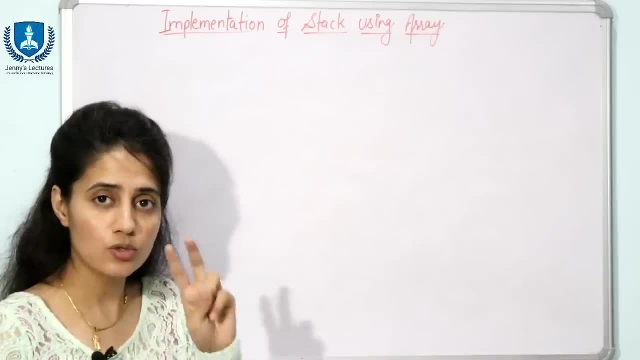 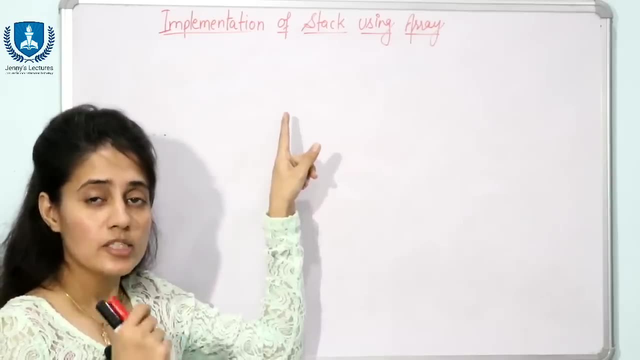 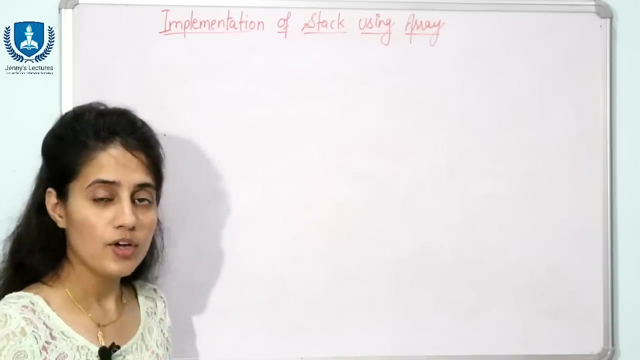 Implement stack using arrays. See, we can implement stack using two methods: using arrays and using linked list. In this video, we will see how to implement stacks using arrays. Means, we will use static memory allocation and we are going to implement all the operations of stack, right. 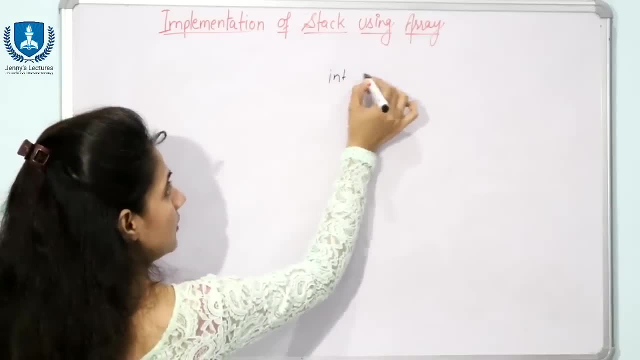 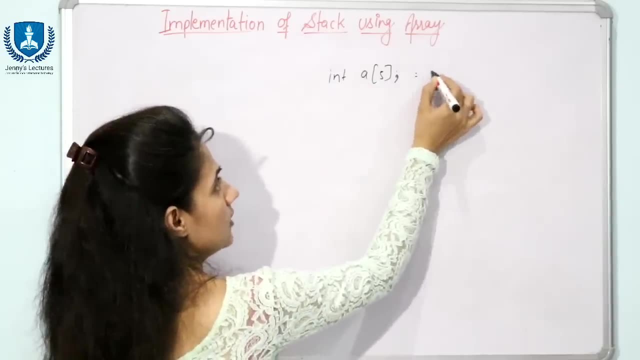 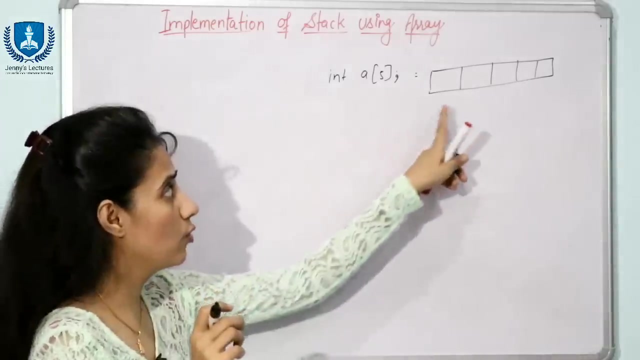 So I guess everybody knows how to declare an array like this: Data type, name of the array and size of the array. right, When you declare this array it means in the memory 5 blocks have been allocated for this array. 5 blocks means how many bytes 5 into for integer, how many bytes For 1. integer 4 bytes would be allocated, Means 20 bytes. 20 bytes would be allocated right. Index is 0,, 1,, 2, 3 and 4, fine, Suppose address is 100, so next this address. for this block address is 104, because 4 bytes for 1 integer right, Next 4. 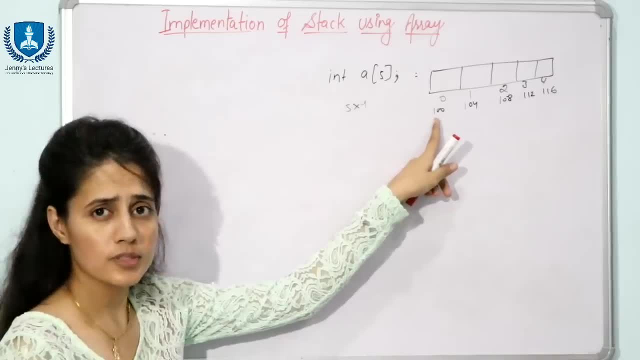 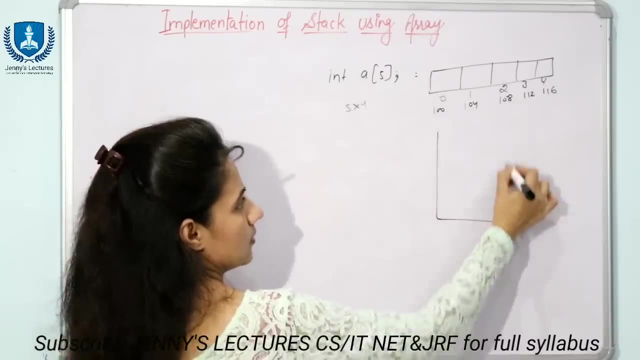 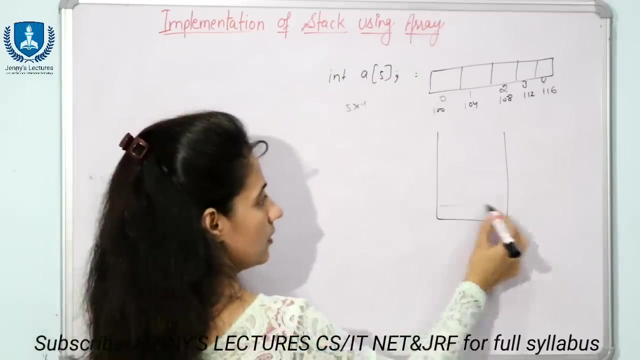 byte for this right. So this is how we are going to represent array in memory. that thing we have already discussed. Now, if you write down this array like this, if you rotate this array like this, it means this is what A stack. this is logical representation of stack. fine, Same 5,. 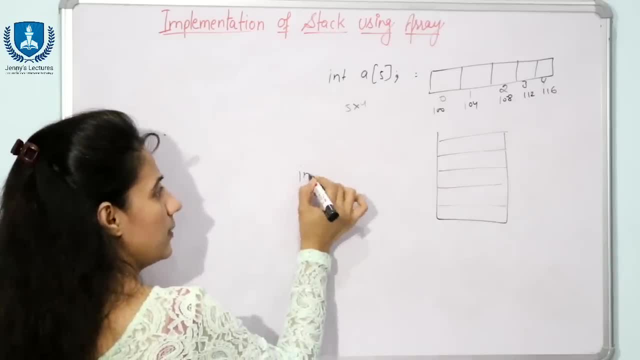 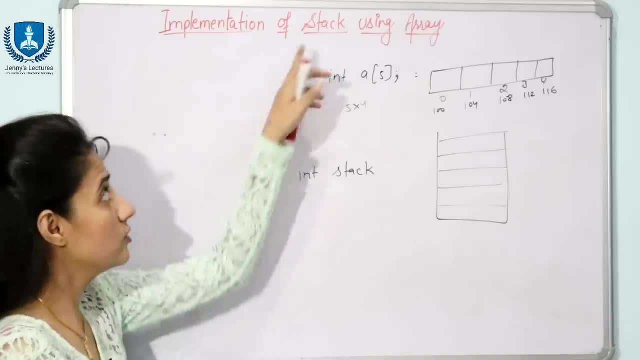 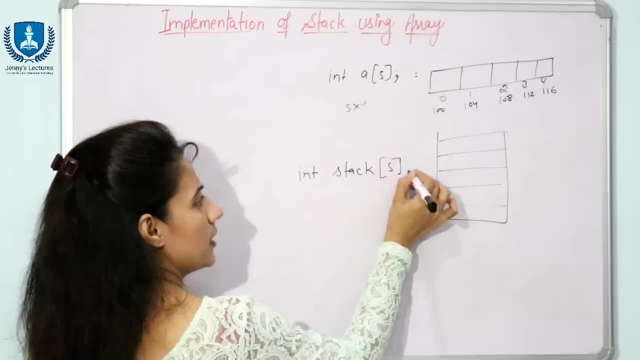 as you wish, right, But we are implementing stack. that is why I am taking name stack. just for an understanding purpose And size, is suppose I am taking 5, right: 1,, 2,, 3,, 4 and 5,. 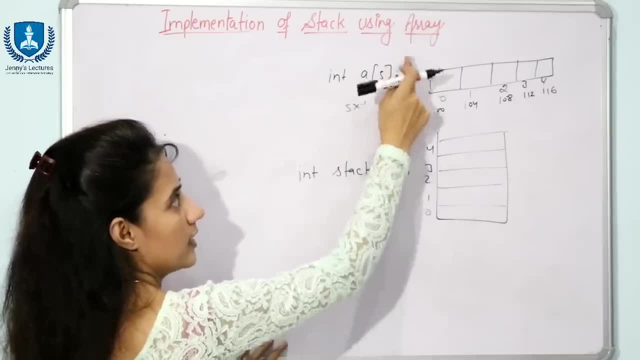 same 0,, 1,, 2,, 3 and 4, because, using arrays I am going to implement this stack Index would be started from 0,, 1,, 2,, 3 and 4, right, So this is how we are going to represent array in memory. 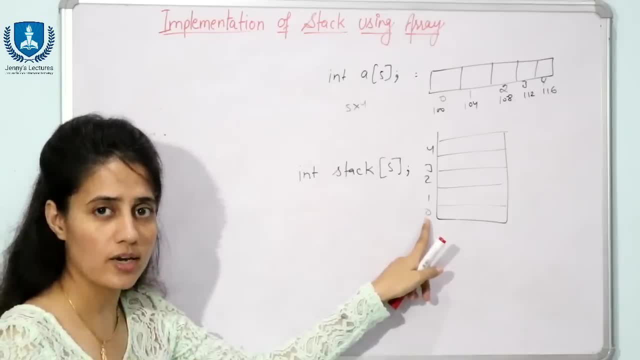 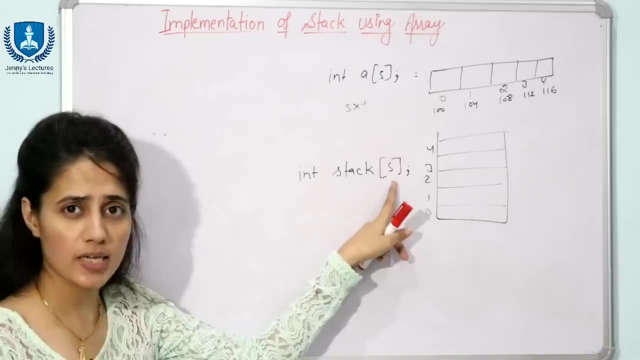 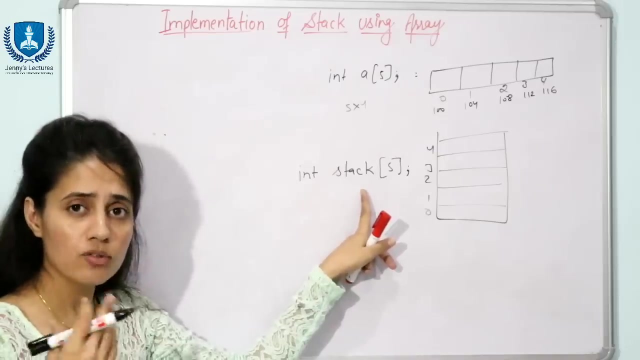 from 0.. We are implementing this stack in c right, So this is how we can declare the stack right Here. we have fixed the size, that is for 5 elements. I want the size in the memory 5 into 4, 20 bytes would be allocated. And now suppose in future I want to insert 10 elements. in that case, 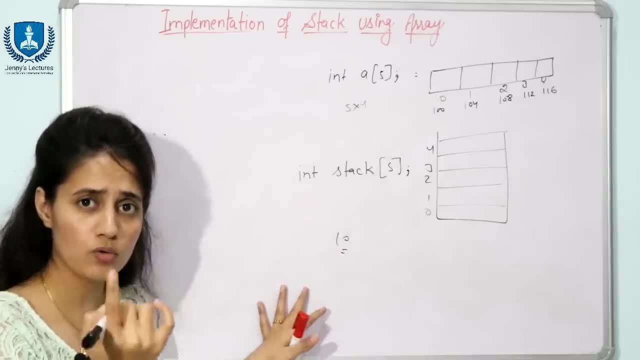 what we can do. The simple rule of array is what Another array would be allocated- maybe of size 50 or whatever. So this is how we are going to implement this stack in c, right? So this is how we are going to implement this stack in c, right? So this is how we are going to implement this stack in c. 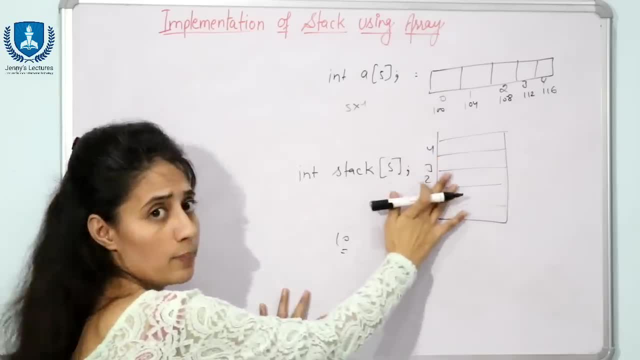 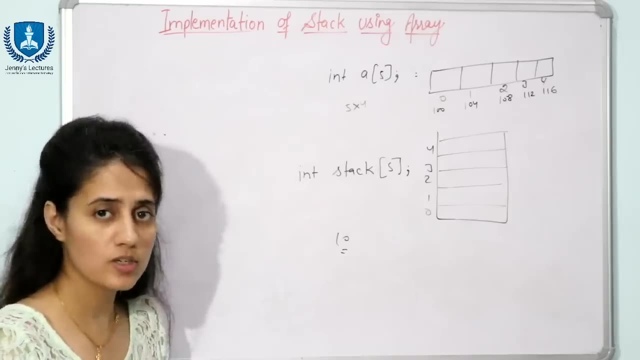 what size you specify of that size and all the element from the previous array would be copied there, and after that you can insert new element there. right, That is what the processor is, because this is what static memory allocation that we have discussed already. when we were 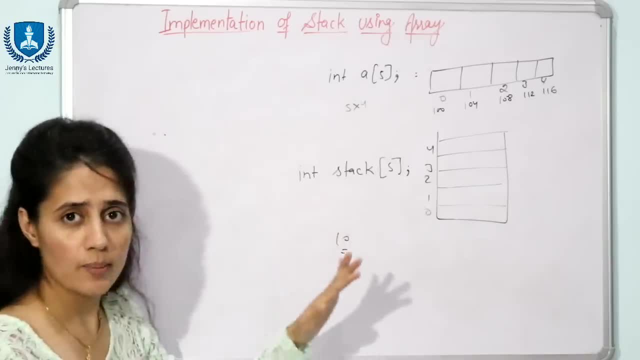 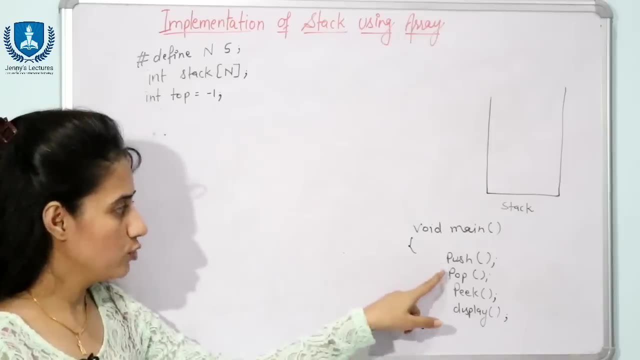 discussing array. Now we will see how to write down a program, how to implement push, pop and all operations of the stack right. So now we are going to define here four function: push, pop, peak, or you can say top or display, or you can say traverse, right. 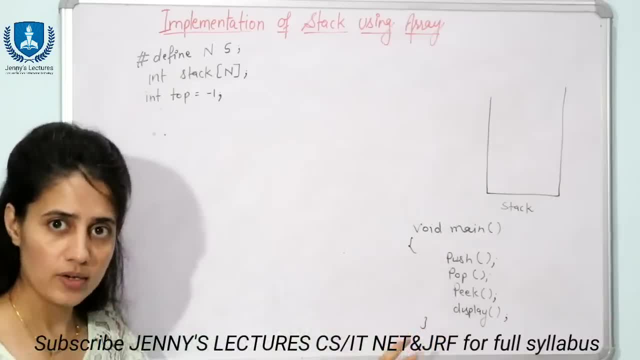 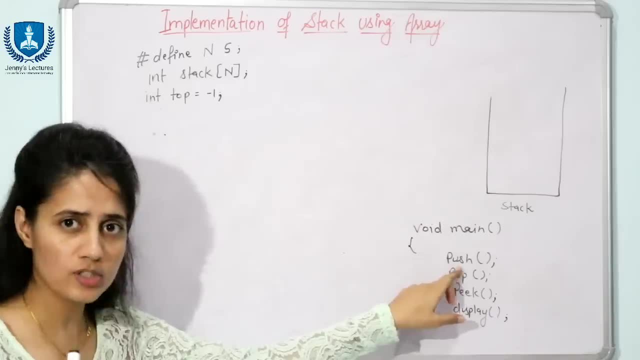 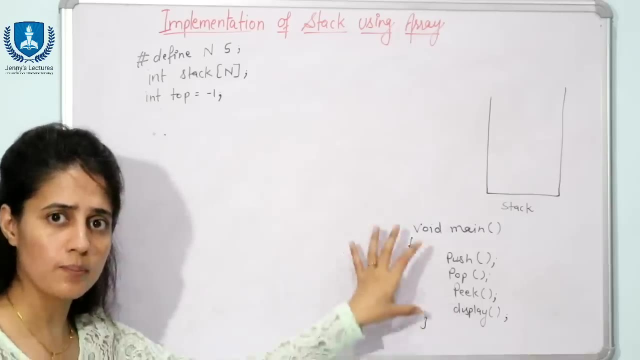 And these function we will call in main function. fine, You can use switch case statements for calling these. function means case 1, press 1 for push operation, case 2 may press 2 for pop, for press 3 for peak and press 4 for display right. Like this you can implement switch case. 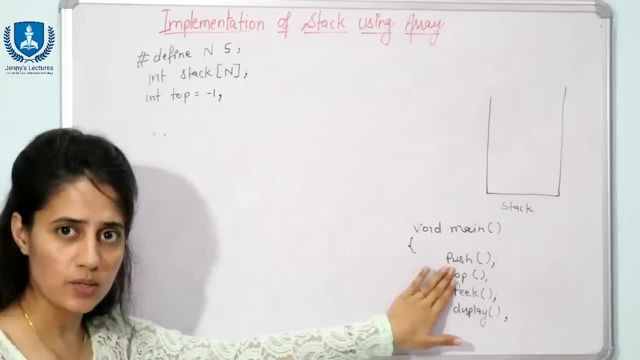 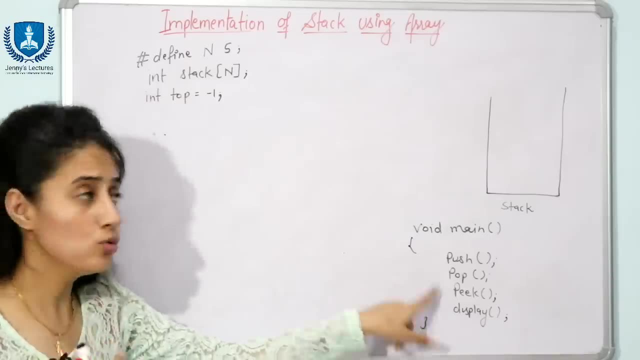 statement. I guess you can write down these function in switch case statement. I am going to implement these function here Now. I have declared here: see in all the functions we are going to use what This top variable. because from the top only we can insert, we can push and delete. or you can say: 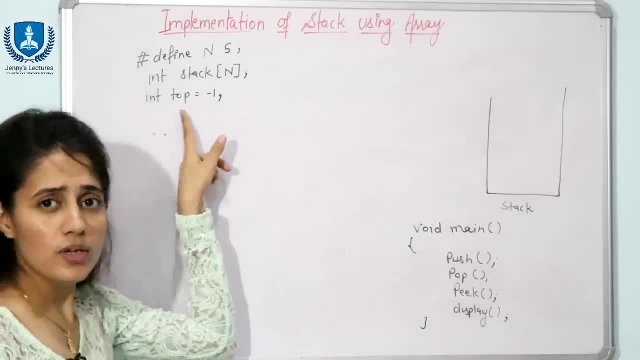 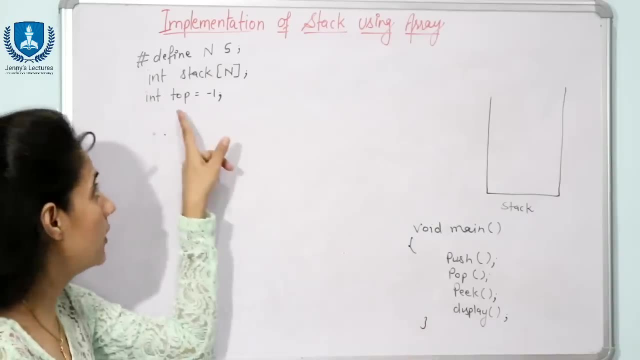 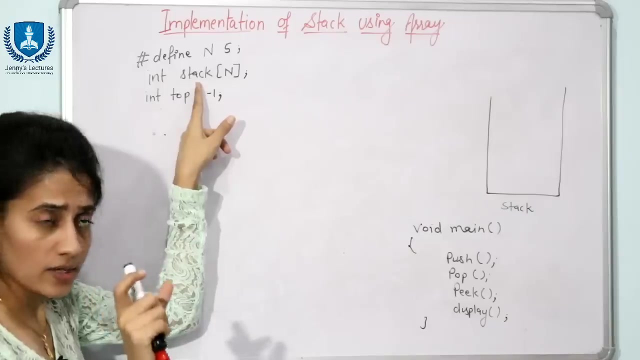 pop element from the stack, right. So initially we initialize what Top is equal to minus 1, fine, And we are going to use this top in all the functions. that is why, globally, I am declaring this variable right And here I am taking int stack. the name is array is stack and here the 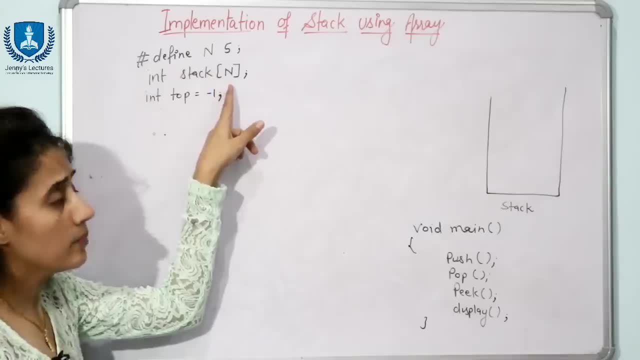 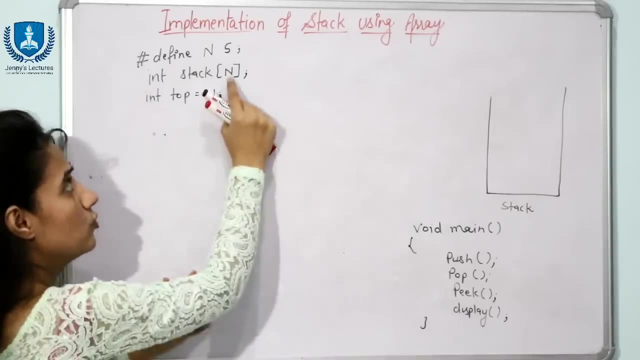 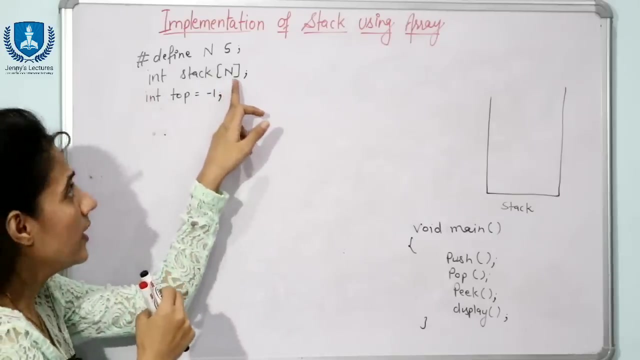 size is n fine. This is what I am declaring globally After header files, outside of all the functions, because inside any function or inside a main function you cannot declare array, something like this. You have to give here constant size because outside. but outside you can declare like this: And now this n is what You can give, this n size. 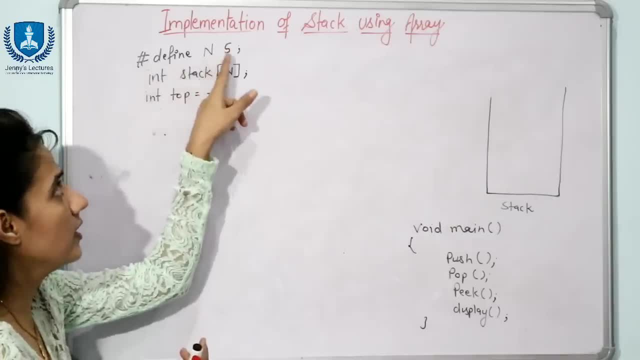 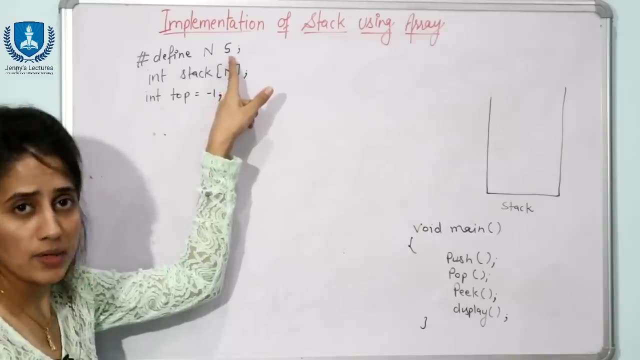 using that macro definition, hash define n. 5, or here you can write 50,, 100,, 500, as you wish. right Means n value can be. here I am taking n value is 5, or if you are not taking macro, then 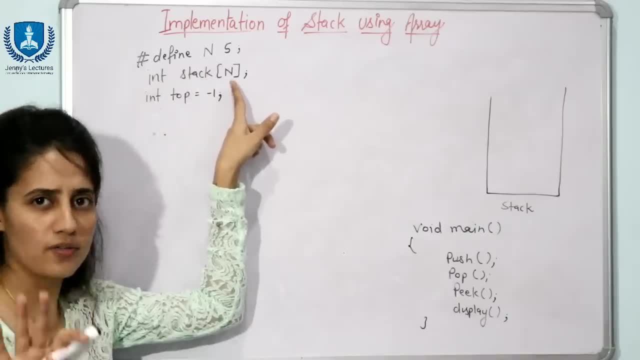 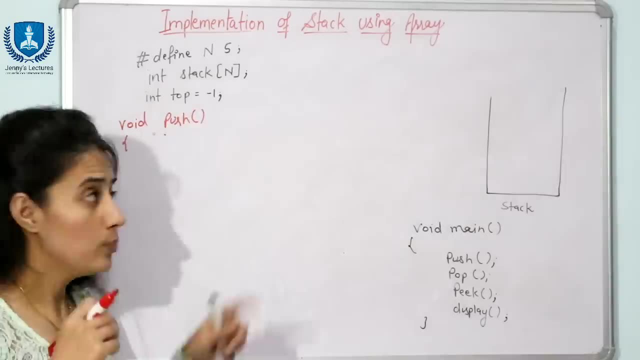 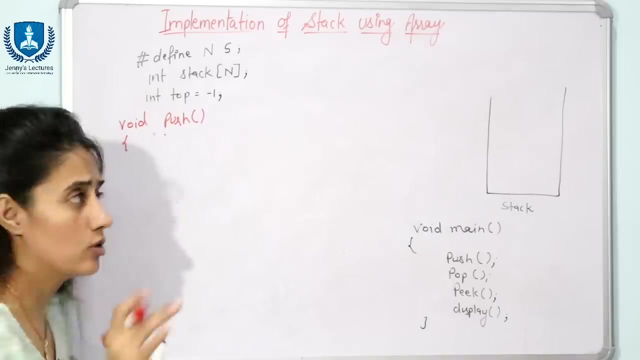 you can write int stack. here you can write size, that is 5.. It's up to you, right. So now, first of all we will define what Push function. So now, in push, obviously we are going to insert the data in the stack. So we will ask from the user which data he wants to insert. So using printf, I can. 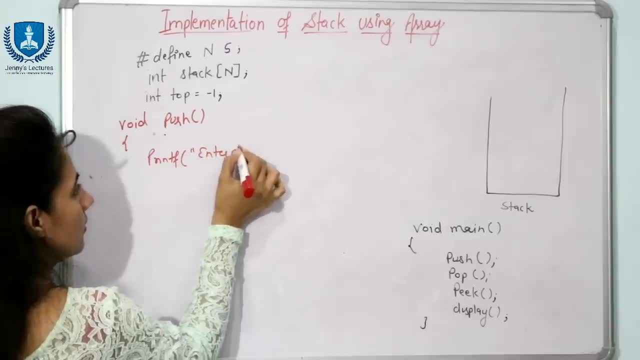 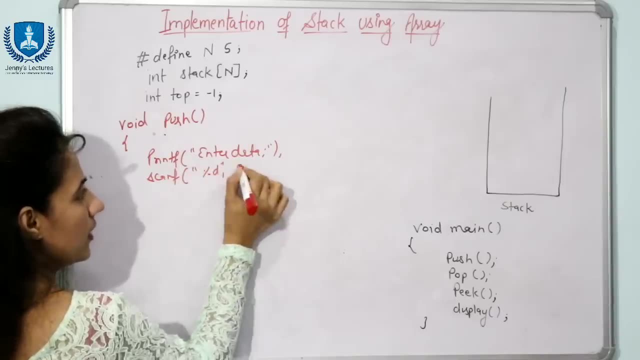 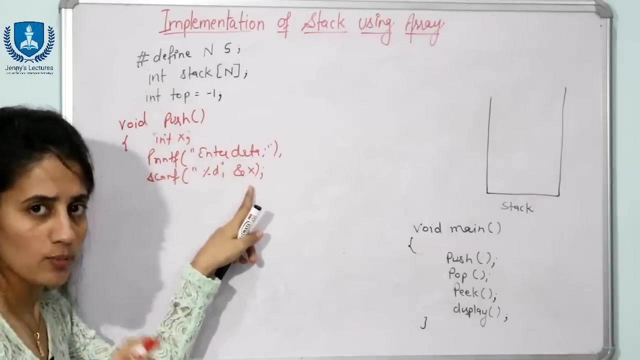 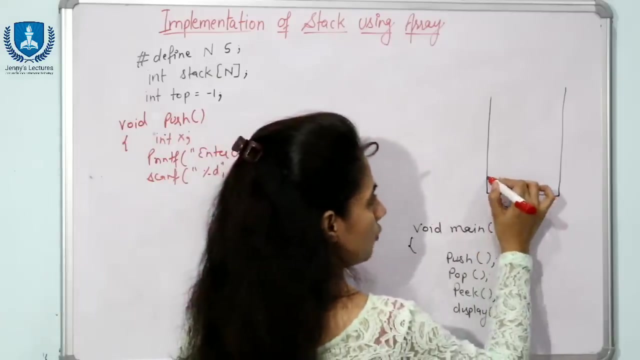 take the value printf, enter data right. And for storing this data obviously you need some variable right. Suppose I am taking x, So in this you have to declare that variable x right. And suppose user has entered here 5.. Now 5 I want to insert here. Now have to insert: See the capacity of. 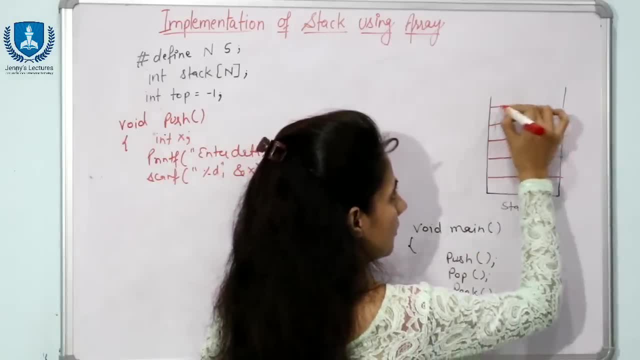 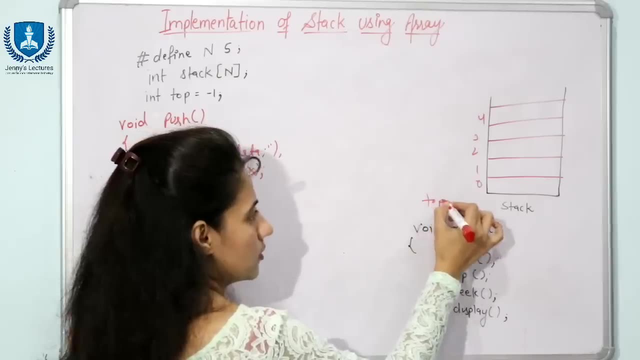 this stack is what 5.. We have already declared 0,, 1,, 2,, 3,, 4.. 0,, 2,, 4.. And top is initially minus 1.. Top is minus 1.. So how to push? First of all, you will increase the stop. 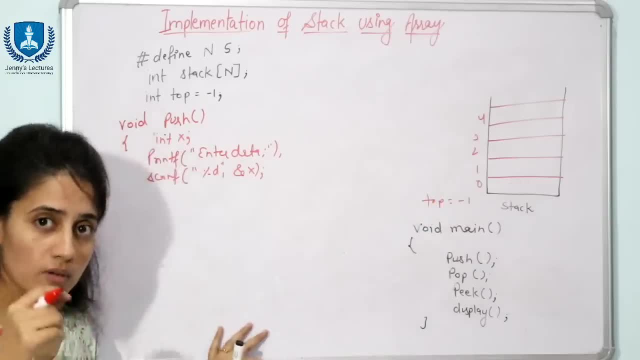 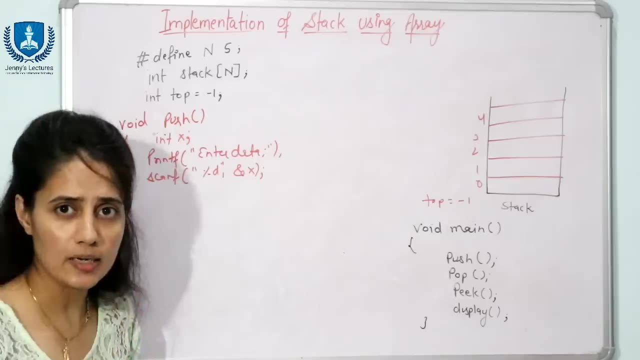 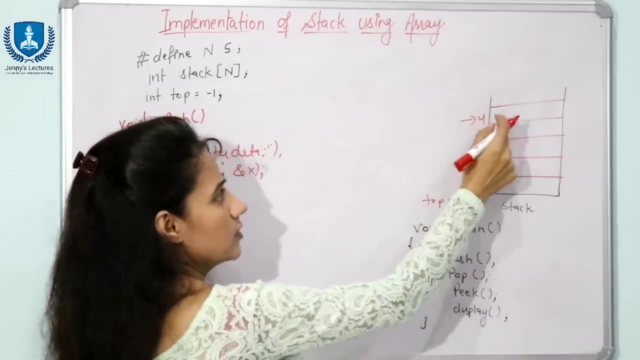 After that you will put here: Fine, But as well as we will check for the overflow condition. If the stack is full, in that case we cannot insert, we cannot push any data. fine. So here first of all what you will write. if now suppose top is here, Top is pointing to 4. Means: here I have 1,. 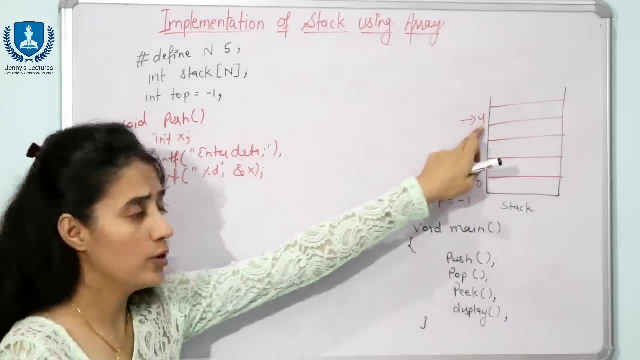 2, 3,, 4, 5.. 5 elements I have. In that case top would be pointing to 4.. In that case we cannot insert any other data here. So what you will write: 0, 1,, 2,, 3,, 4.. So here top is 1, 2,, 3,, 4.. 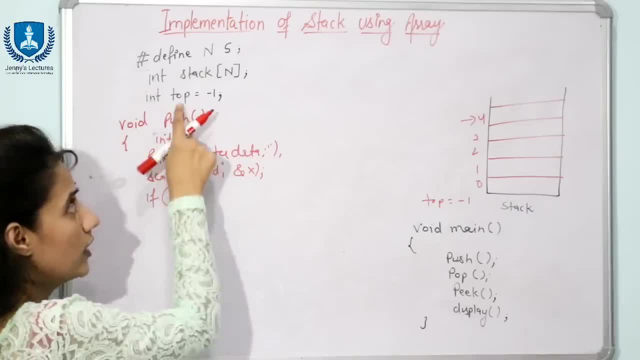 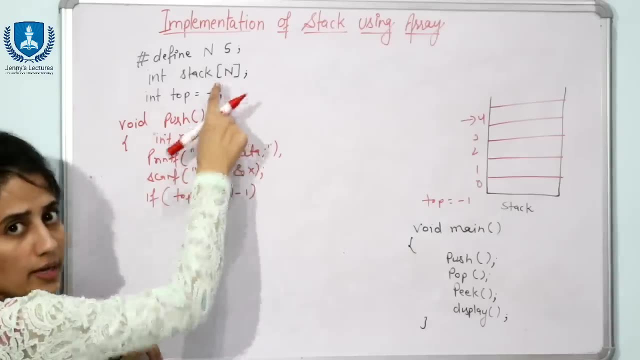 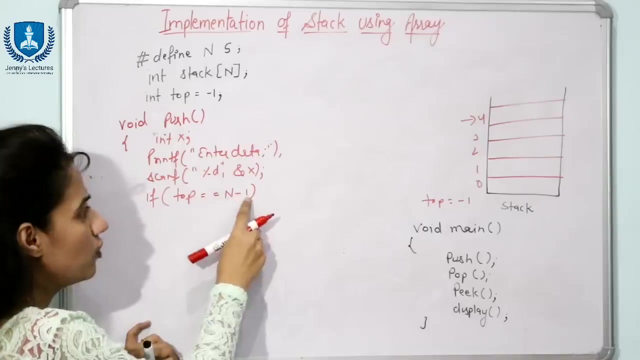 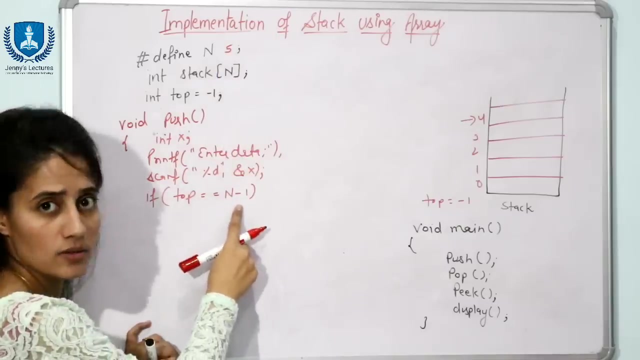 write in if, if this value, the top is equal to, is equal to n minus 1- see here i am taking what n you can simply write. if you take directly here 5. so here you can write: if top is equal to, is equal to 4, here n minus 1 means n is 5, 5 minus 1, that is 4, right. so if top is 4, in that case 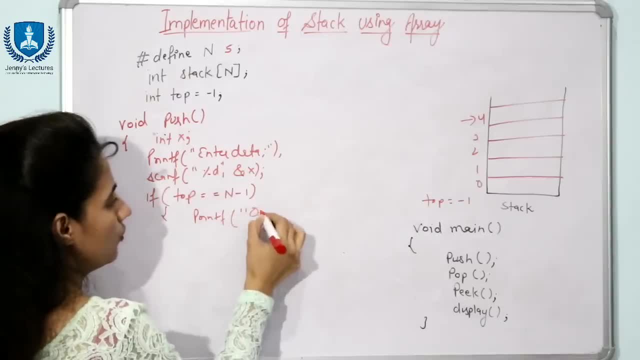 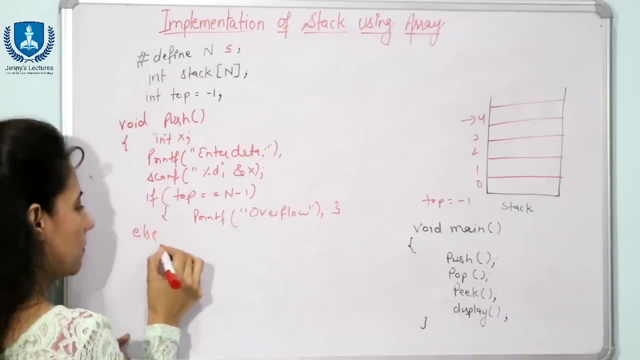 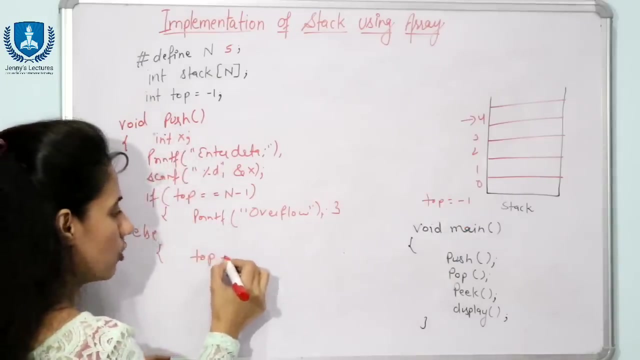 here you can print overflow condition. you cannot insert right else, else you will do what now? first of all you will increase this top. first you will increase top plus plus, or you can say top is equal to top plus 1. after that you will insert the data. so here now. 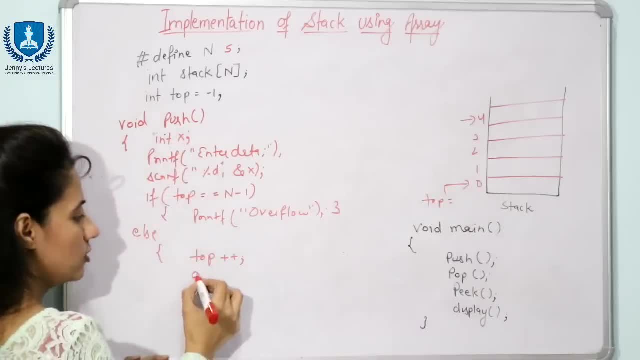 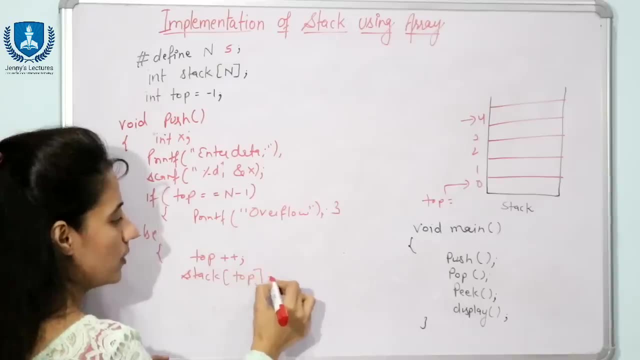 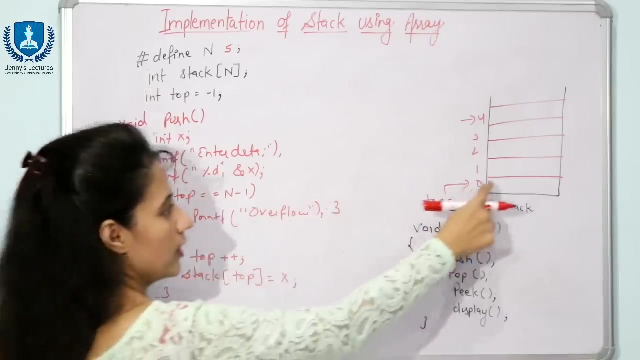 top is equal to 0 here now. now you will insert: see array name is. here I am taking stack, not a. now stack of top is equal to x. top value is 0 means stack of 0. here I will insert x. suppose x is 5, so here I will insert. 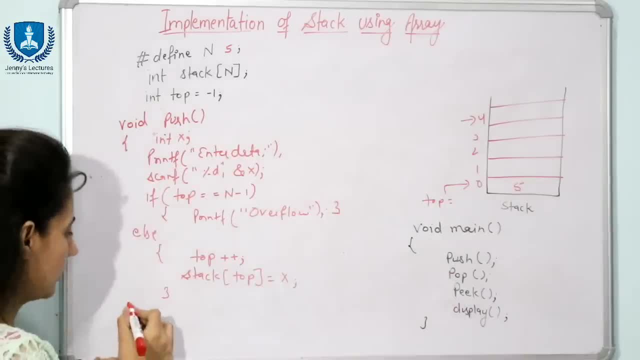 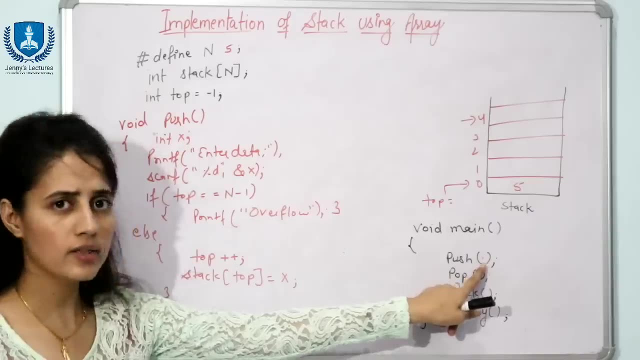 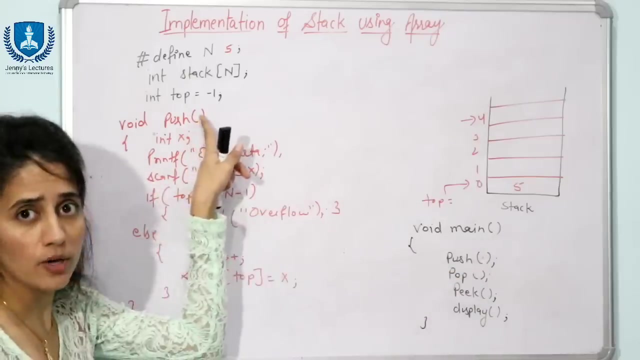 5, right, and that's it about this push operation. or here, if you will not ask the data here, if you want to pass the argument here, then here directly you can pass: right, push, push, maybe 5. you can pass here. you have to receive that value. so void here push and here also you need to write down that. 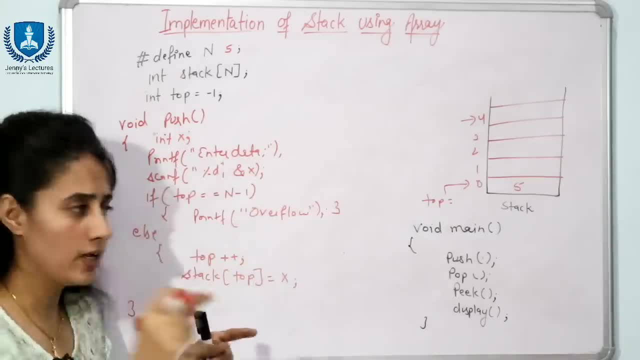 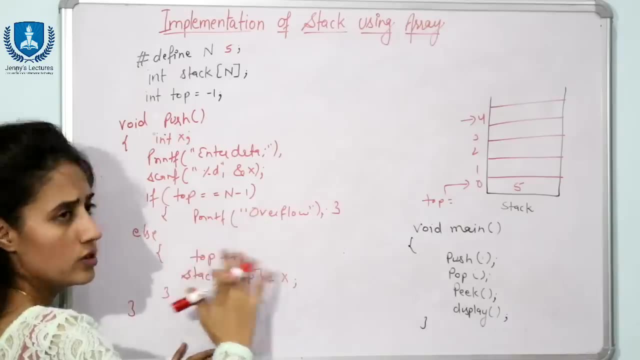 int of any variable name, like int x or int a, where you can receive this value. fine, and no need to ask, no need to write here printf and scanf directly. you can write down these statements right here. you can write down that variable name you have taken here. fine, so here. second method is: you can. 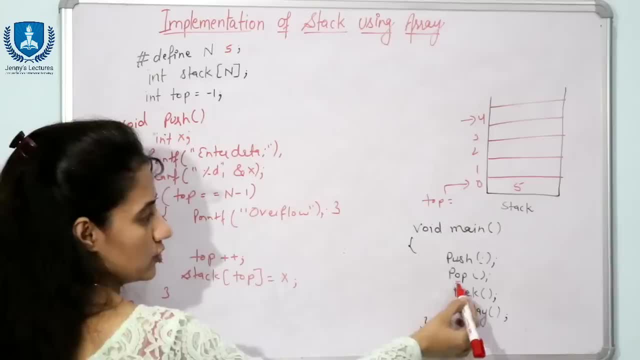 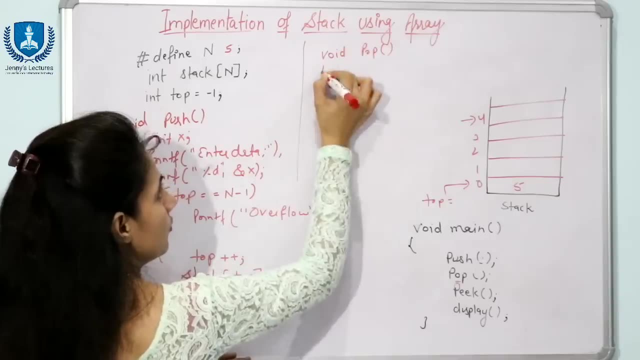 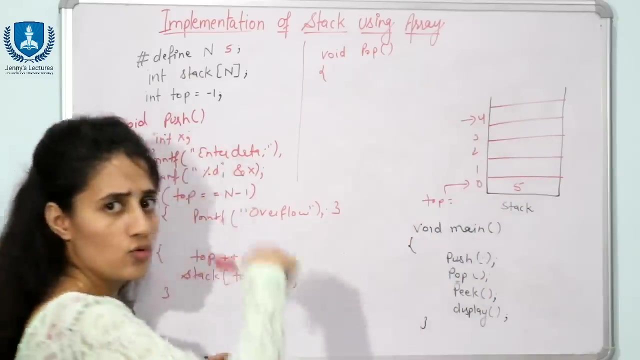 pass the value in the argument. so now we will define this function pop, right here I am writing this coding, I am writing void pop. we are not going to pass any argument in pop that I have discussed already when we were discussing that theory part, that in pop always the top element would 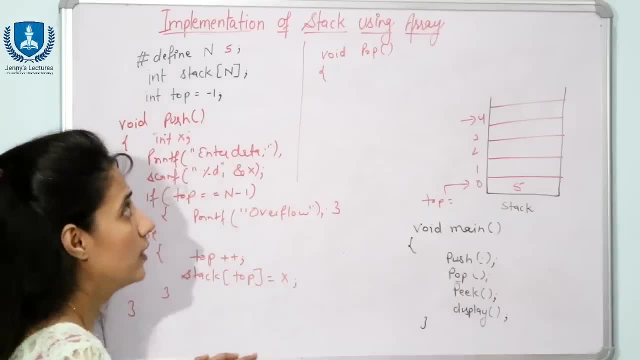 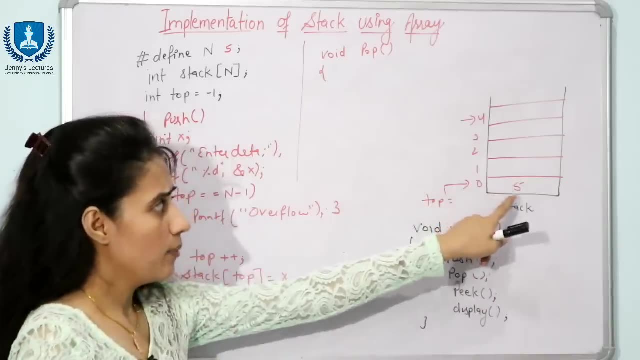 be popped out, so no need to pass any argument here. fine, now, if you want to print that value, that deleted value, suppose here the top is 5 only I have only one element and I want to print that value. so here the top is 5, only I have only one element and I want to. 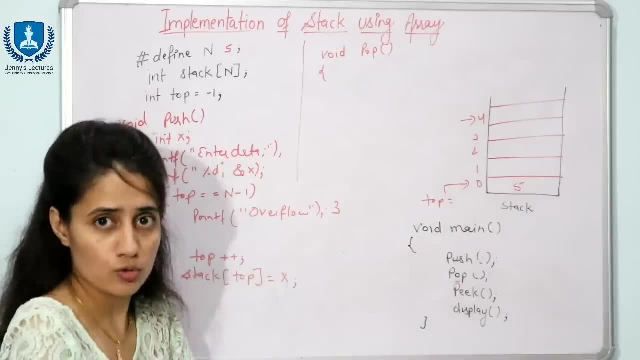 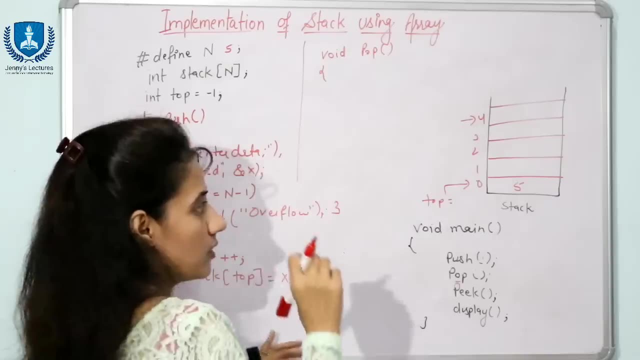 a new domain and I want toumps this a 5 only. I have only one element and I want toبح to pop this and i want to print this value also. fine, that the popped item is five. fine, so in that case, what you will do, see simply in the pop. you will do what top minus, minus as you. 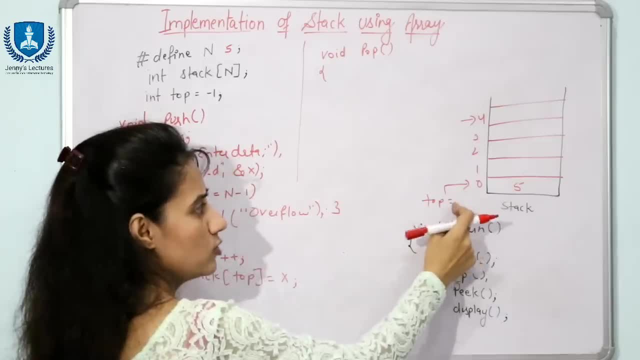 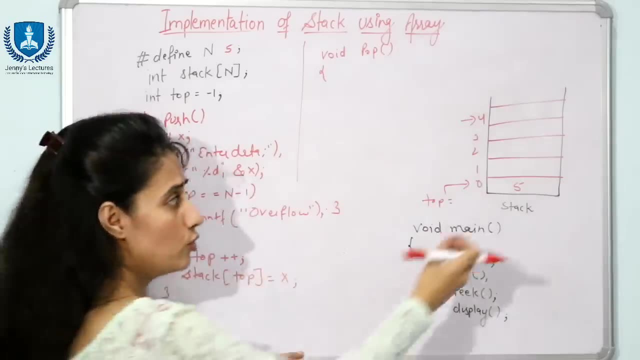 have discussed in previous case. after that, top minus minus means top becomes minus one and this is now the garbage value. no need to delete this value. or if you want to print this value, in that case first of all you will take out this value right, store this value in some another variable. 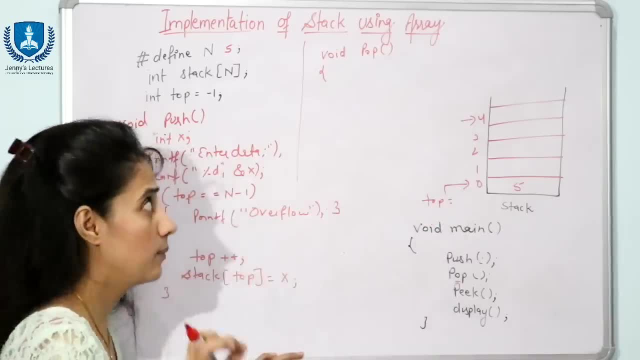 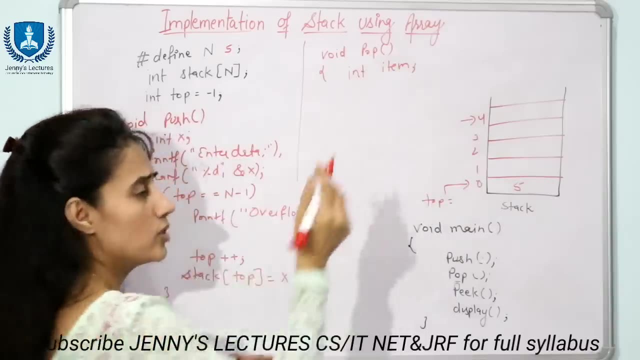 after that you will do top minus minus and after that you can print that variable. now, what you will do, see obviously, for taking out this value and for storing this, we will take another variable, that is suppose int item- i am taking fine- and you will also check for underflow condition if there is no. 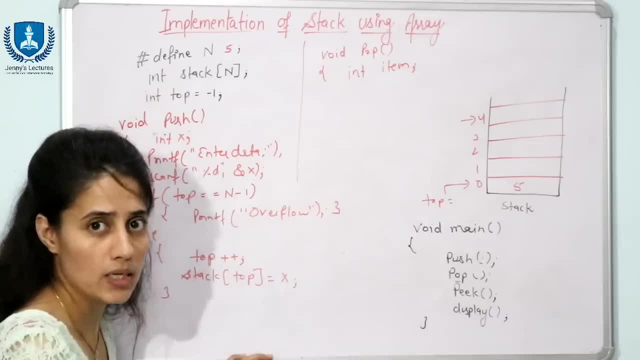 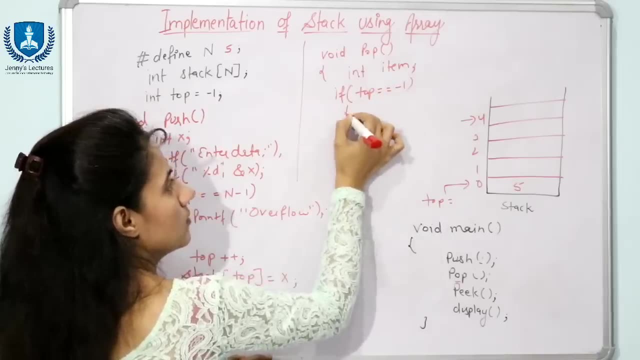 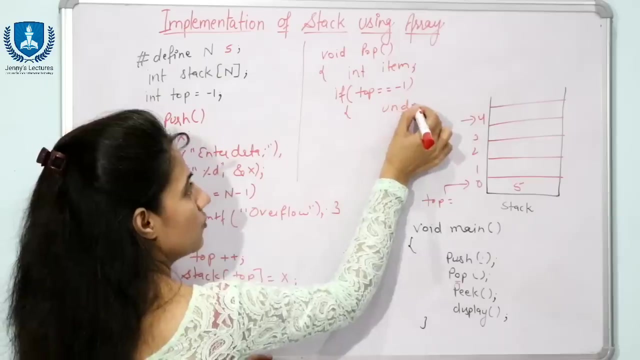 data in this stack, then you cannot pop anything that is under flow condition. so what you will write? if top equal to equal to minus one, fine, if top is minus one, then no data is there in the list. so here you will print simple underflow. in printf you can write underflow else. 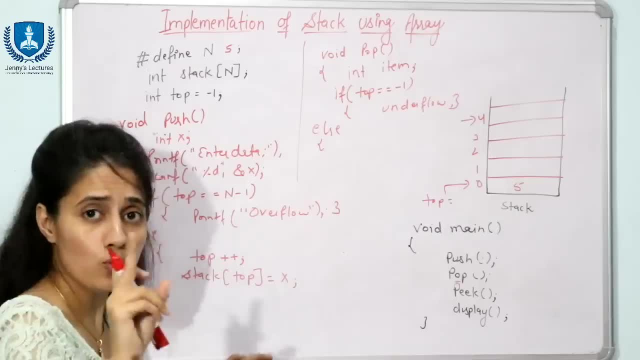 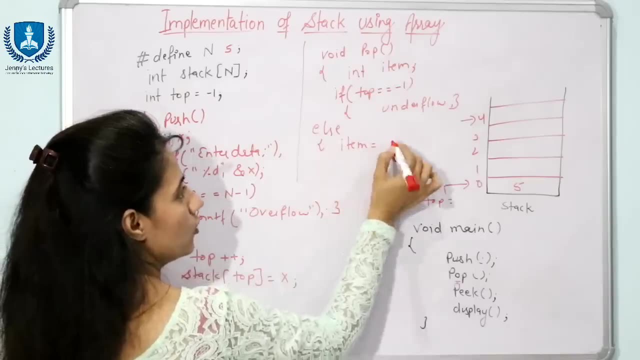 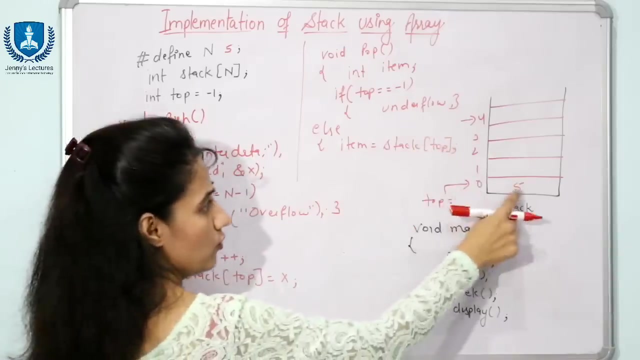 else, first take out this value if you want to print that the popped item is this one. so first of all, simply take out this value. store this in item. item is equal to stack off top right now. stack of top itself means five has been stored in this item now. 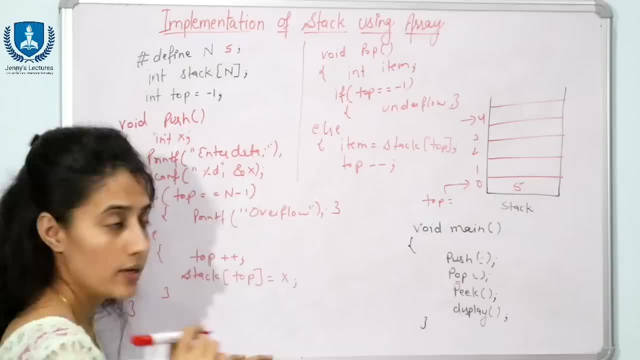 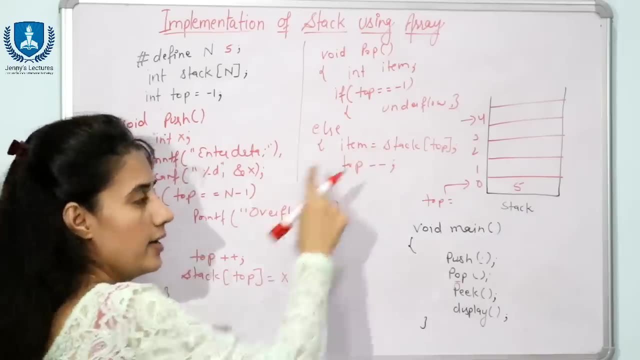 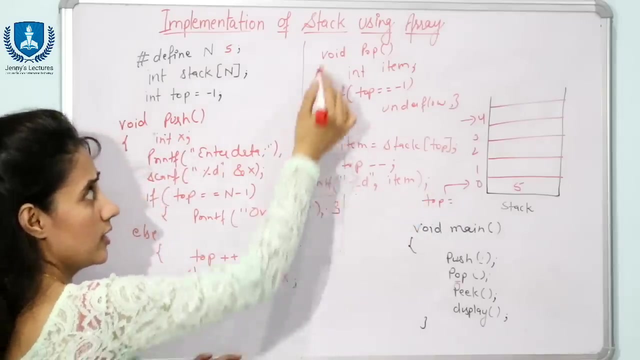 now you can do top minus minus, right, and here you can print that the deleted, the popped item is percentage d and item. so like this: here you can print printf: the popped item is percentage d and here you can write item and after that you can close this else and then this pop function right. 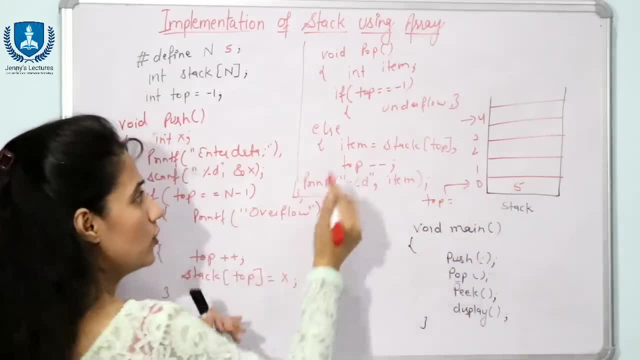 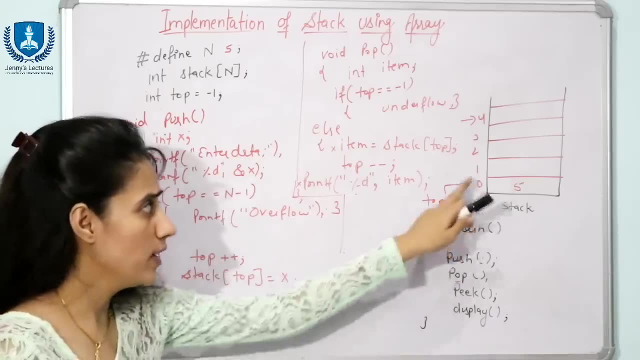 and if you don't want to print, this are the illusions, but later go ahead and road so you can want to print this popped item. then simply what you will do. no need to write down this line. simply do top minus, minus and no need to write down this line. fine, if top minus, minus top would. 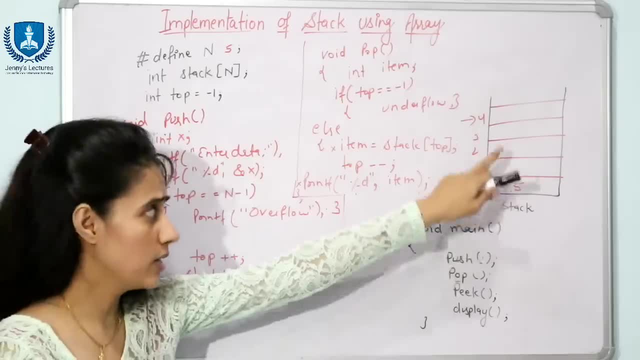 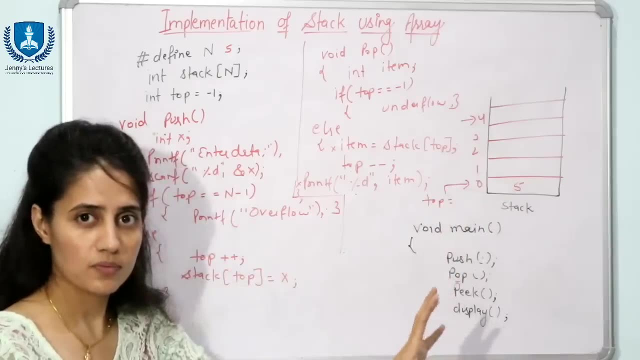 be minus one, that this value become garbage, and we don't care what garbage lies here, because after that, when you will push any other other data item, then this value would be overwritten. that is fine, right. so now this is push and pop operation. now we will see what is peak operation. so, as we have, 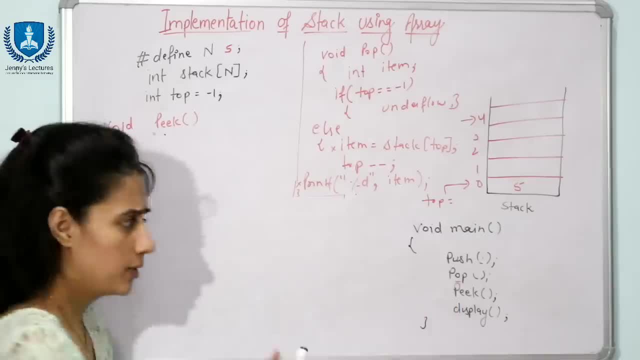 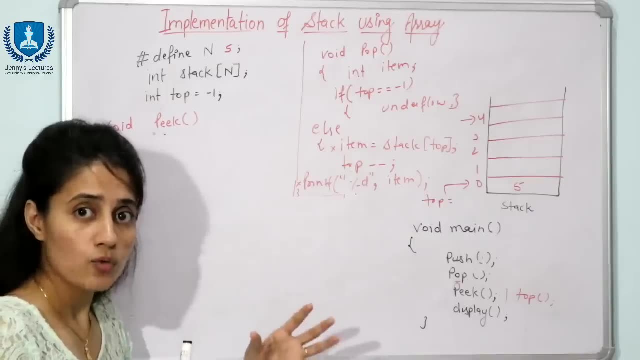 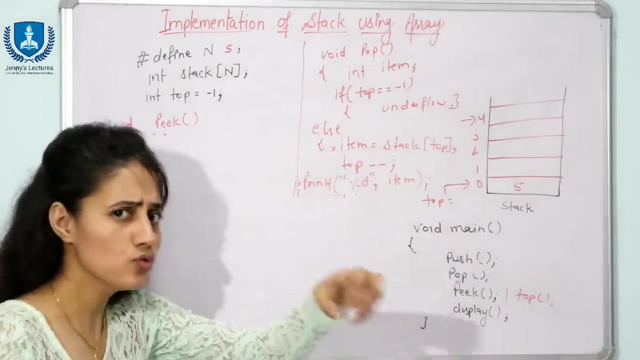 discussed in the previous video. what is this? peak operation or the top operation? you can say top. top element means getting the top most element of the stack without removing that element from the stack. right means without doing top minus minus. i just want to check out which is the top. 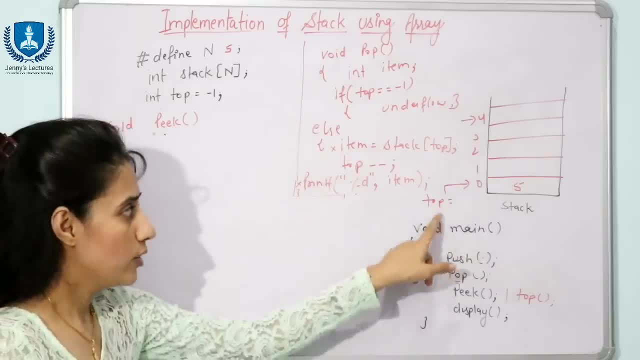 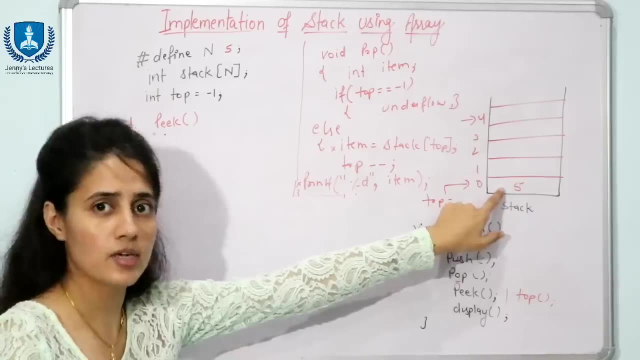 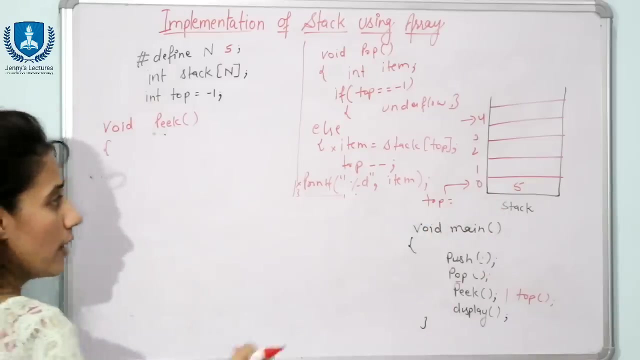 most element of the stack. that's it, right. so here, if you call this peak, it means it should return five. but we will not do top minus minus. this five would still be in the stack. we just want to see which element is at the top of the stack. right, so how you will print. 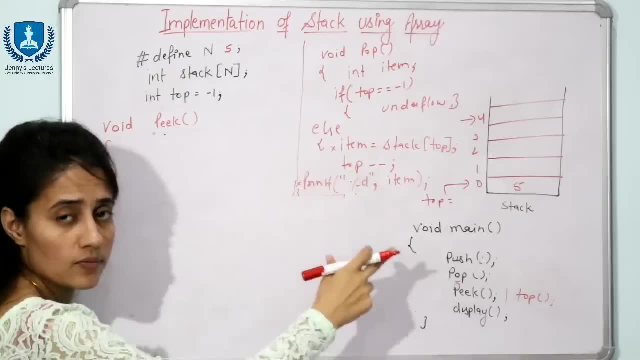 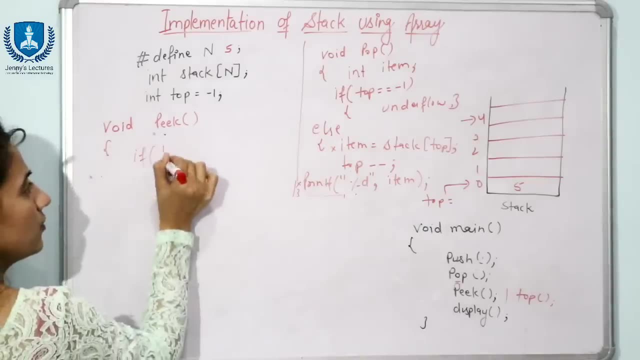 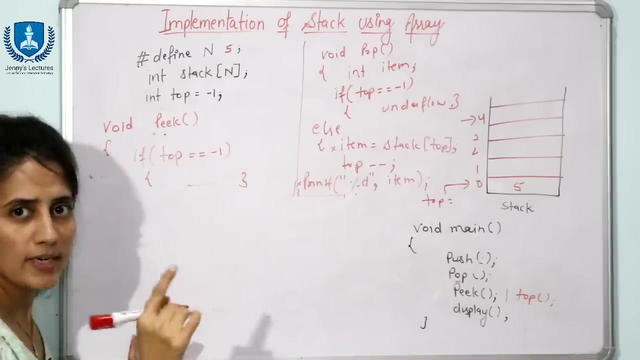 that thing. so now, if in the stack there is nothing, then the top most element is there is no element in the list, so it should print stack as empty. so how you will check if top equal to equal to minus, one same thing it means here you can print what print: f stack is empty, right else? 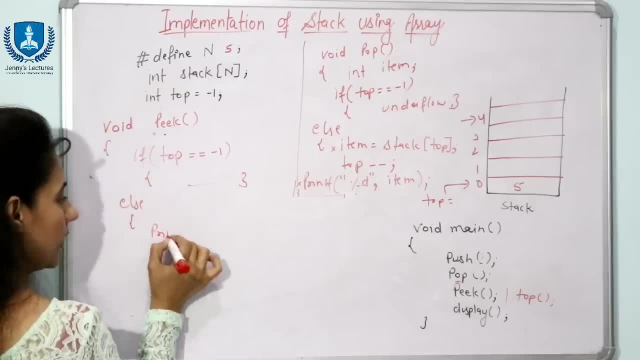 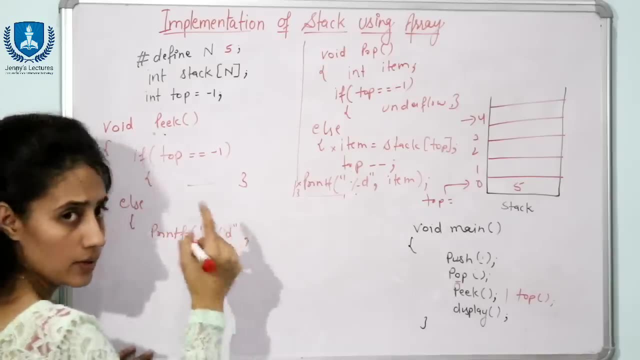 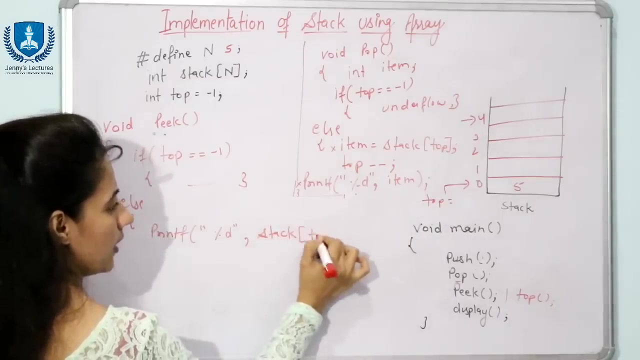 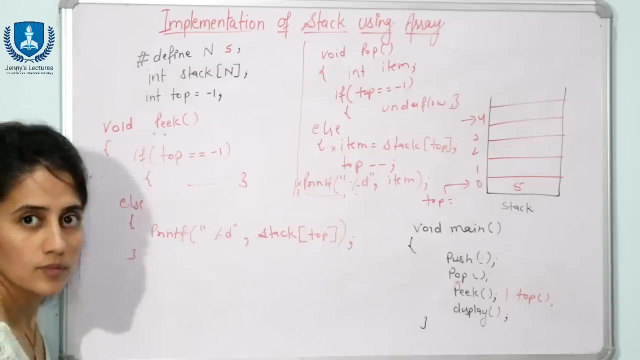 you will print the top element. so here, simply, you will write: print f. the top most element is percentage d. after that, here the top most element. how to print name: here i am taking star and here you will write in subscript: top, the top element. right, in this case, top is now zero because only. 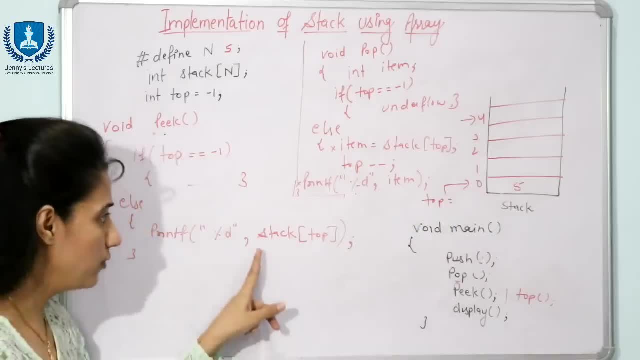 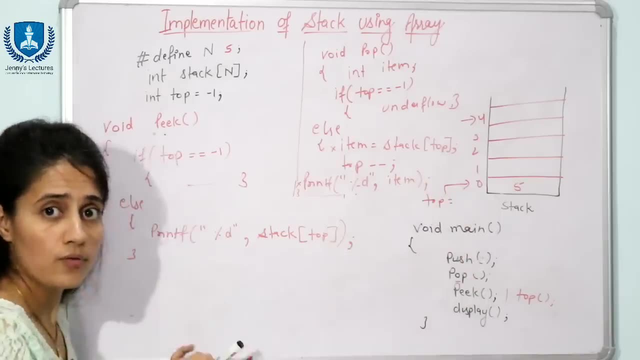 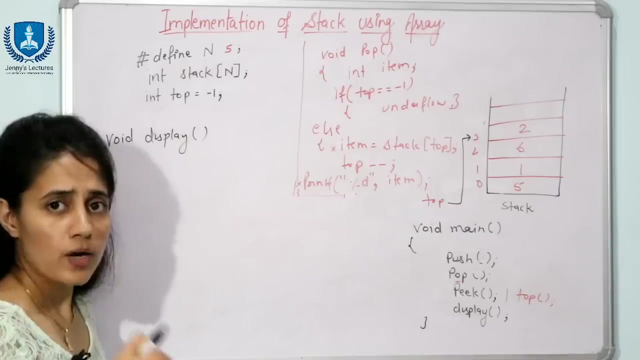 one element is there, so five would be printed. and here we will not do top minus minus, because we are not going to remove this from the stack now. this is the peak function. now we will display the content of the stack. or you can say: we are going to traverse the stack. fine, suppose we have called this push function four times and 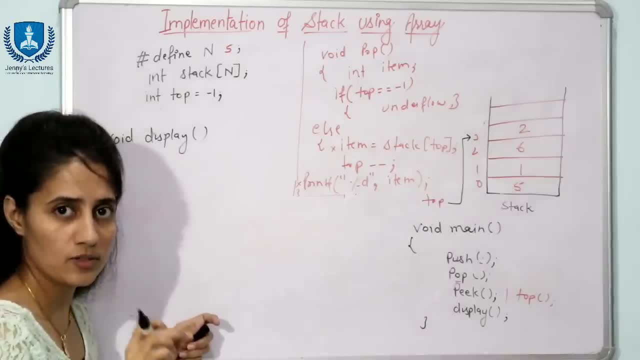 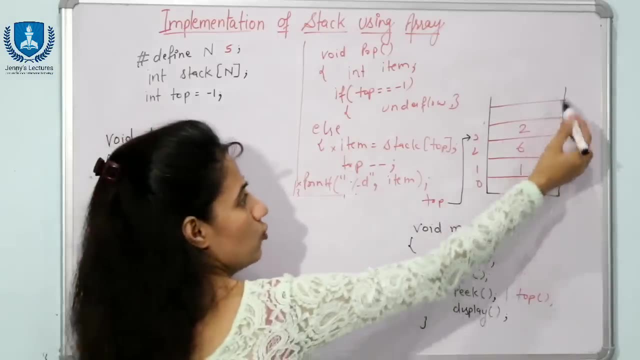 five, one, six, two. this is now the stack. these are elements in the stack. fine, now i am going to traverse the stack. i am going to display the content of the stack. so here, first of all, we will display two, then six, then one, then five. they are not popping out, we are just displaying the content, or somewhere. 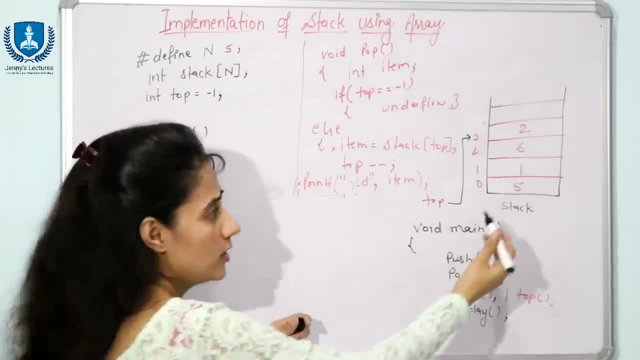 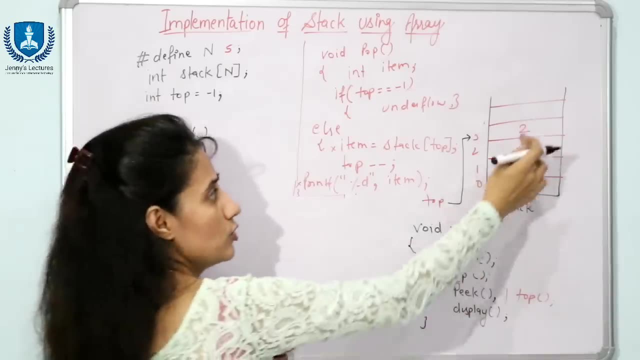 you also find out that they will start the loop from here. only they will display five, one, six, two. and somewhere you find out that they will display two, six, one, five. it's up to you. here i am going to display from the top of this, this one, because we cannot, we. 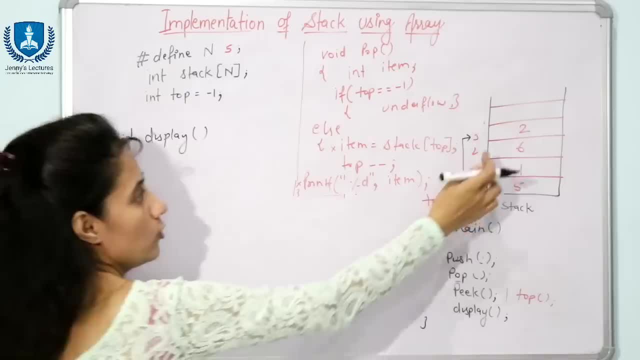 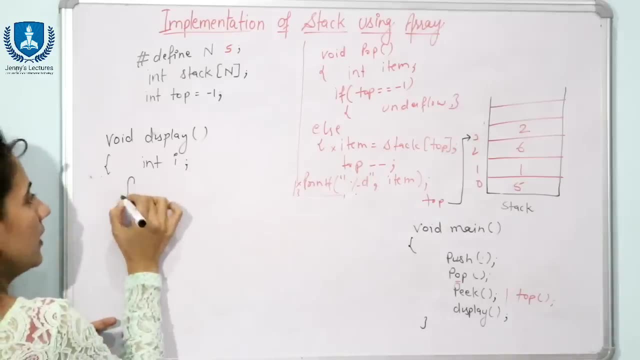 can access from the top only fine. so now we are going to start a for loop. obviously right. for that we need a variable. suppose i am taking here i and here i am writing a for loop, here, here and here i have: i equal to an, i great, equal to i, the whole Nonен, i has all the. 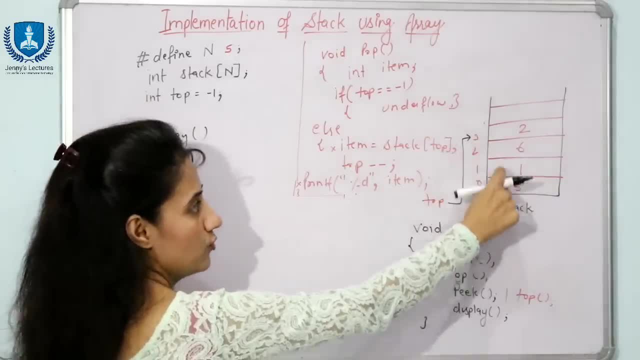 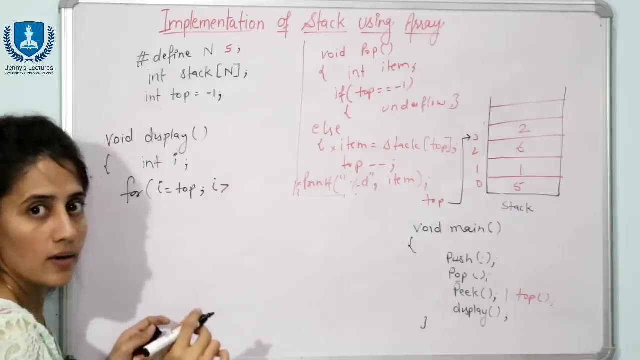 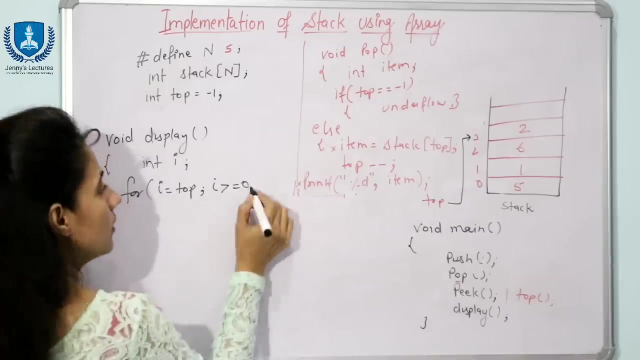 data back. but i can't get to the i in the change. so after pushing the cheering Rabbit image, if i want to print, that may look like that. if i want to write, i, i, i. it's better to just to name the material. but this is out time because it takes time to type in wanted. to print the answer in the data a, and this is what i will do. i am going to print i, the value variable, the, the variable that i will use. i am going to print a difference. oh, sorry, i want to print x, so i want to print here. then i am going to print: i is equal to i, such thenける. 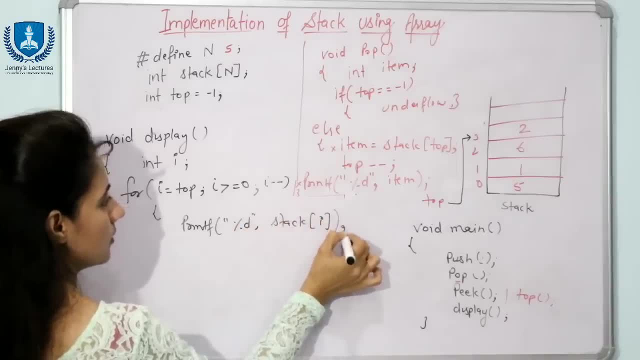 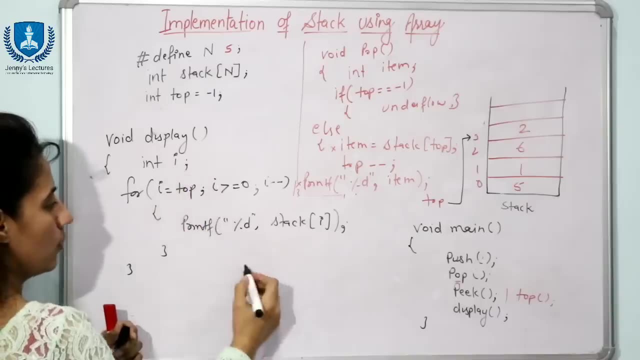 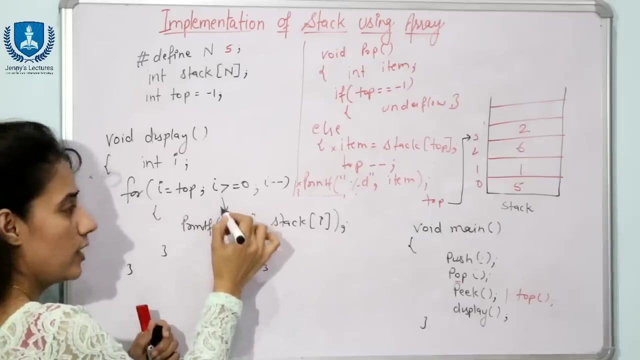 and stack i. right now you can traverse this thing. i is equal to top. now i is equal to in. at this case, top is equal to 3, so i is equal to 3. 3 is greater than equal to 0. yes, so control will enter. 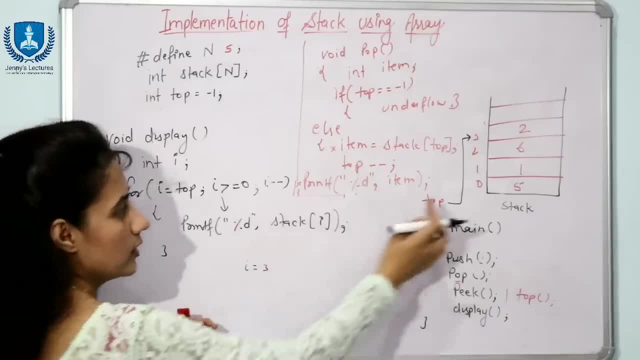 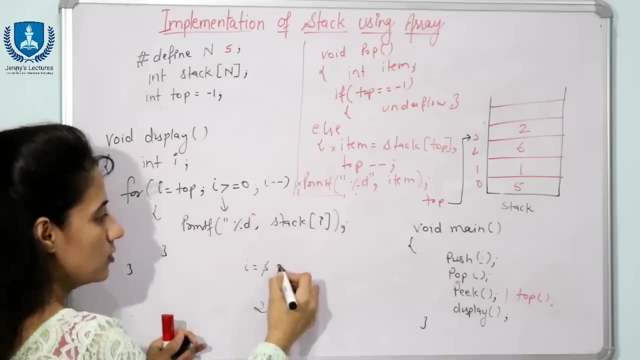 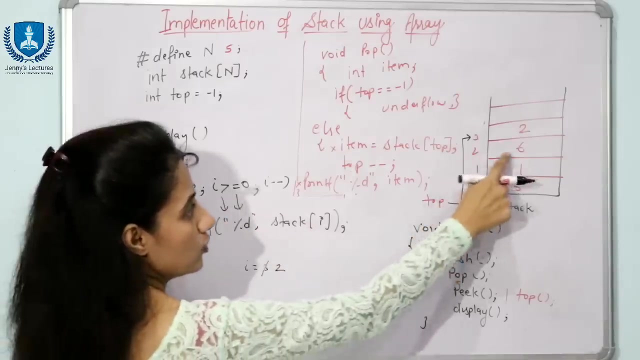 into this loop printf: percentage d stack of i. stack of 3. in stack of 3 i have 2, so 2 would be printed. right again, i minus minus, now i becomes 2. 2 is greater than equal to 0. condition is true. control will go into this loop. stack of 2 would be printed. stack of 2 is now 6. 6 would be printed. 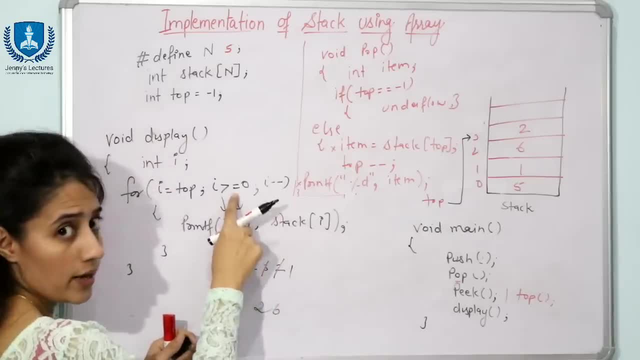 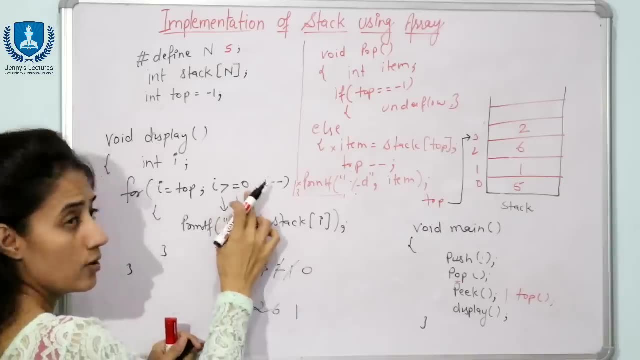 i minus minus, now i becomes 1. condition is true again. now what would be printed? stack of 1. stack of 1 is 1: 1 would be printed minus minus 0. 0 greater than equal to 0. condition is true again. enter into this loop. stack of 0 is 5: 5 would be printed. 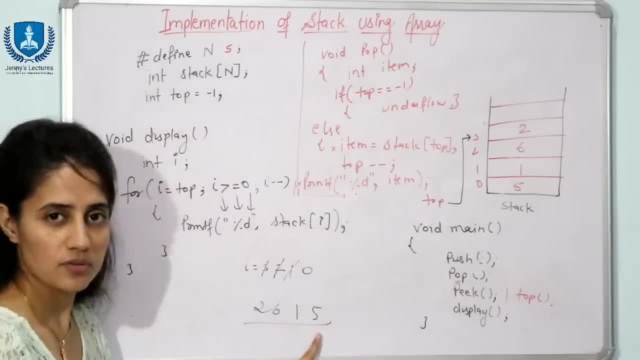 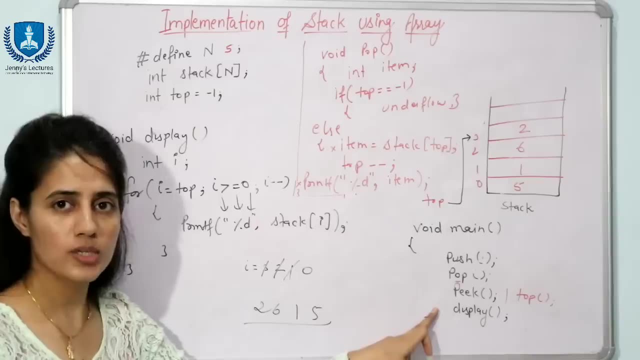 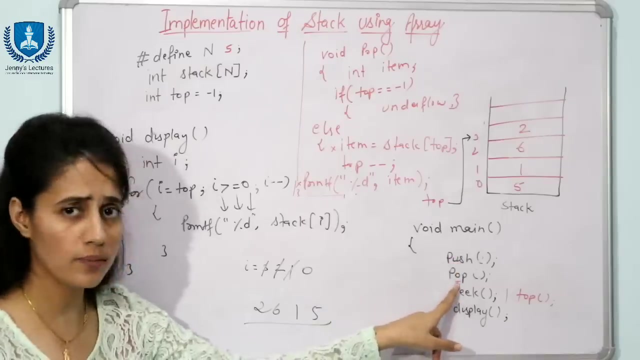 now this is the output: 2, 6, 1 and 5. right, this is how we are going to traverse the list, traverse the stack, and these function you will write in switch case statement. i guess everybody can write down these thing in switch case statement. case 1 means push then break. case 2 means pop then break. 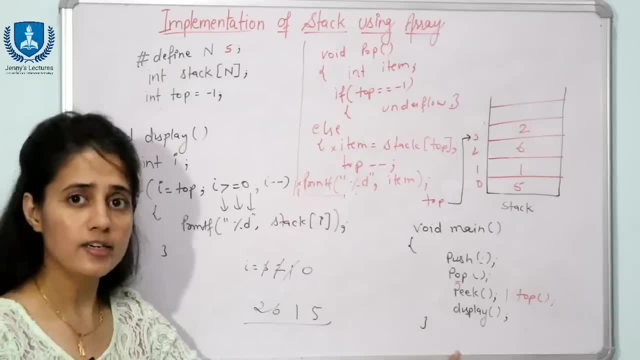 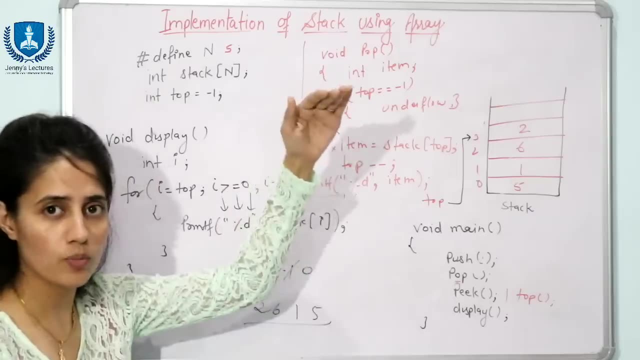 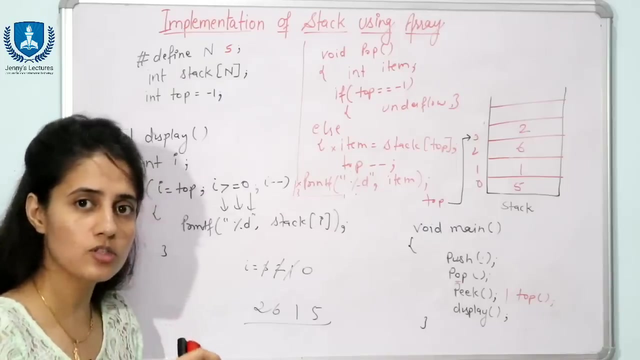 case 3 means peak, then break. case 4 means display, then break, and in default case you can write down invalid choice. and you can write down the switch case into do while loop. fine, and condition may be: while choice not equal to 0. if 0, you will press 0. it means exit. right, see, this is how you. 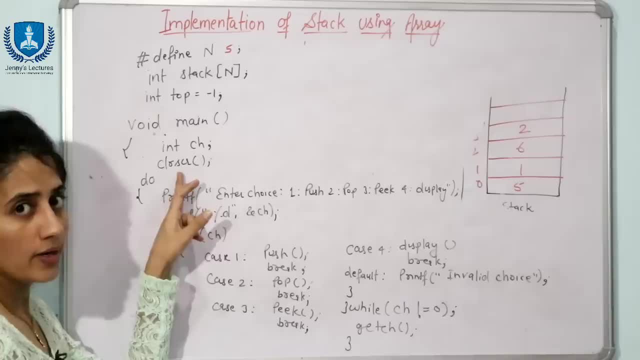 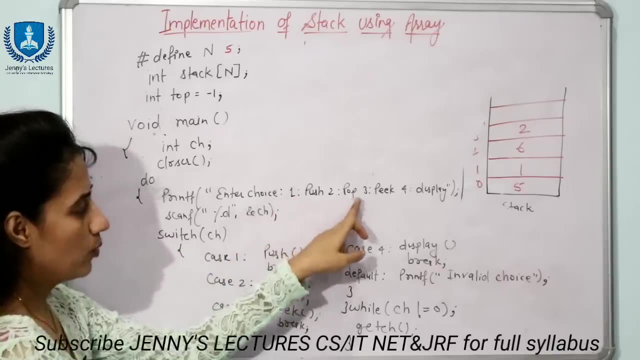 can write down the main function using the switch case statement right using do while loop, do and do while loop. i am taking here fine enter choice 1 for push, then 2 for pop, 3 for peak and 4 for display. i am taking a variable ch where i am taking the choice from the user. so i am declaring: 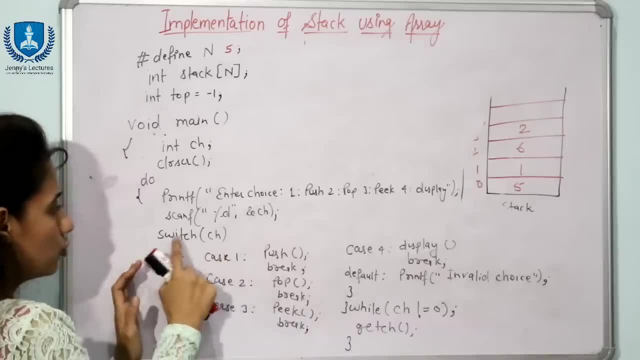 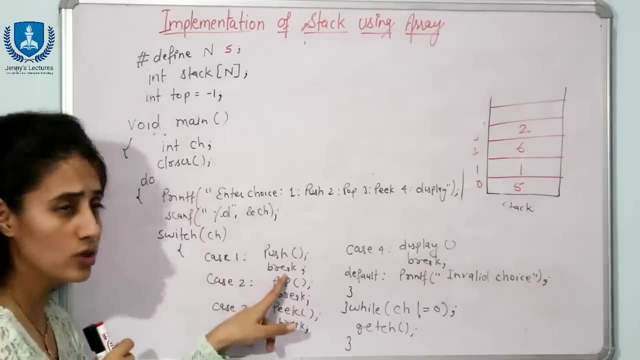 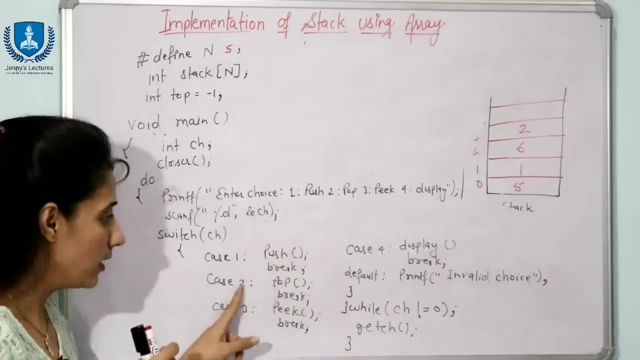 that variable here. fine, this is for clearing the screen switch here. i will pass that choice. in case one, i will call push. when you will press one, then push should be called, and after that you are using break. see if you do not write this break. in that case, if you will press 1, then push should be called, after that pop would be called, right. 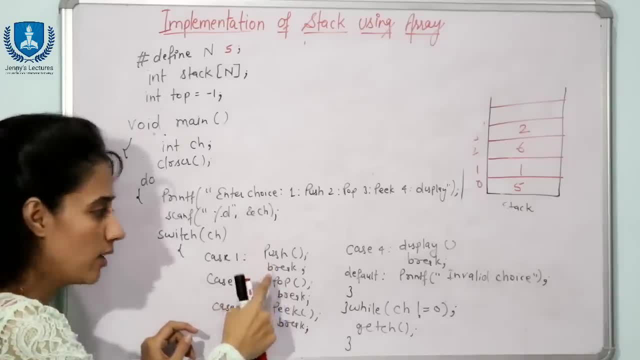 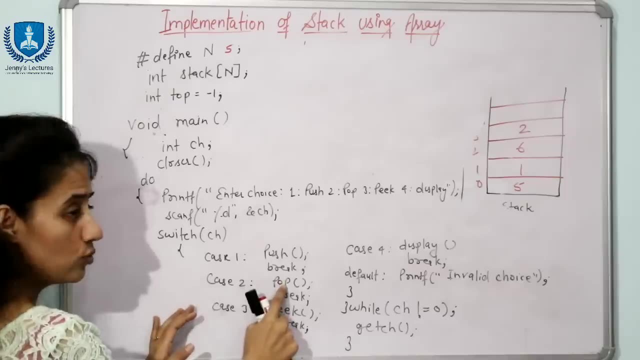 and if you will use this, break means only push function would be called and after that, break means again it will ask to you for the another choice, right? that is why we are using here: break in case 2: we are using we are calling pop, then break in case 3: we are calling peak. 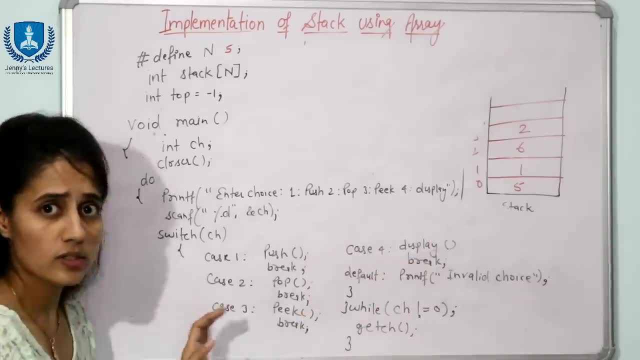 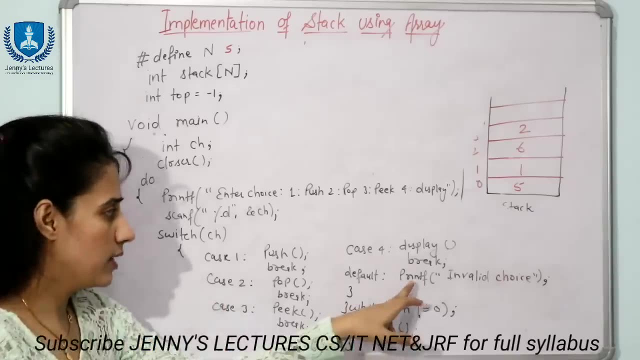 then break. in case 4 we are calling display and then break default. suppose if you press 6 in that case, i want it should print some invalid message. i mean proper message. that is why i am taking here: in default case, printf is equal to invalid choice. when you will enter 5, then it will print invalid. 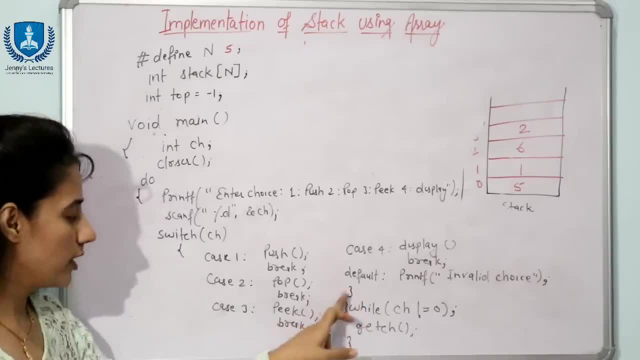 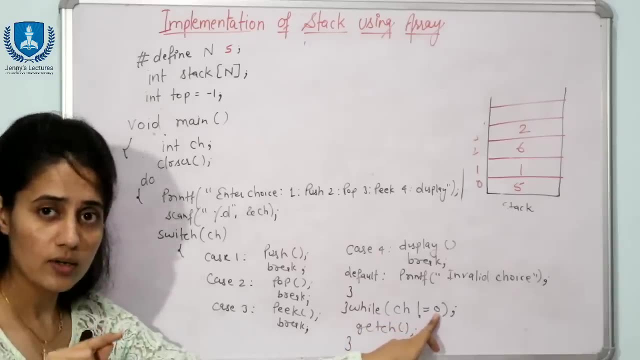 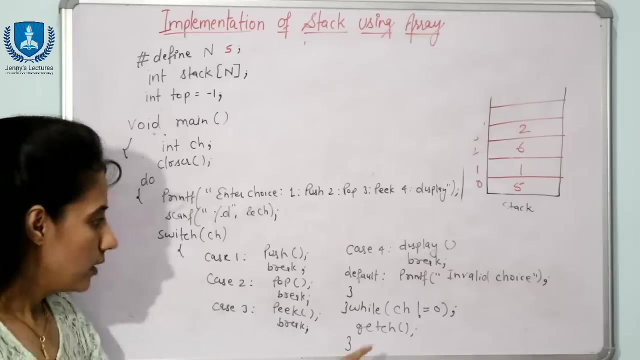 choice right after that closing this switch and after that closing this. do while choice not equal to 0. it is what? 0 right, if you will press 0, means you will. you are going to exit, fine, from the output screen and then get cs. this is how we are going to write down that main function. i guess everybody. 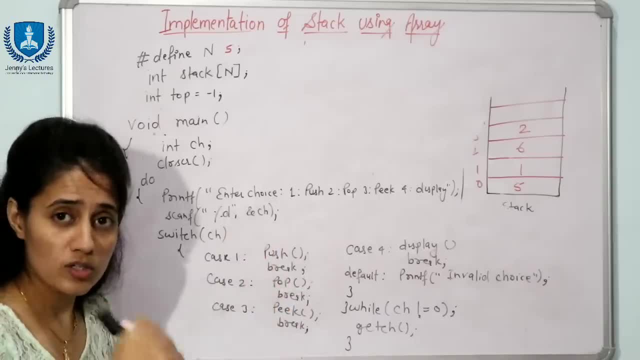 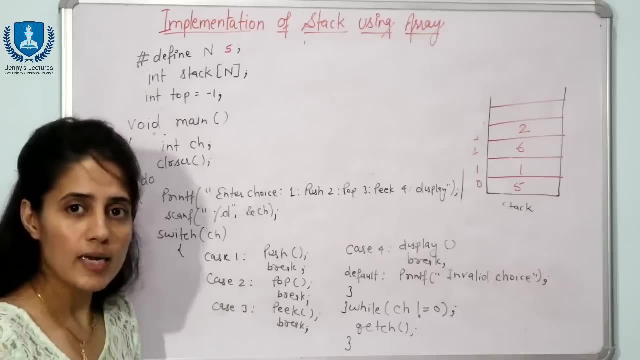 know the syntax of switch case statement. fine, so this is how we are going to implement the stack using arrays. in next video we will see how to implement stack using linked list and all these operation- push, pop and this peak operation, all these operation- is going to take how much time. order of one. 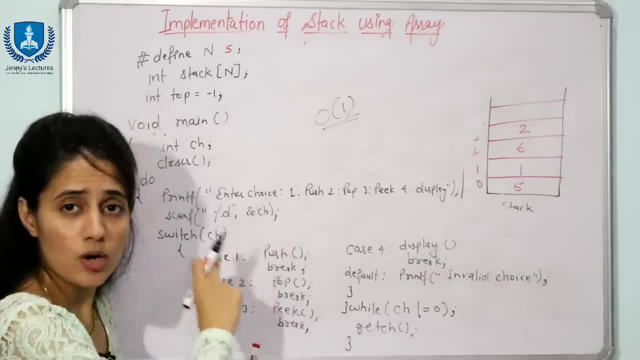 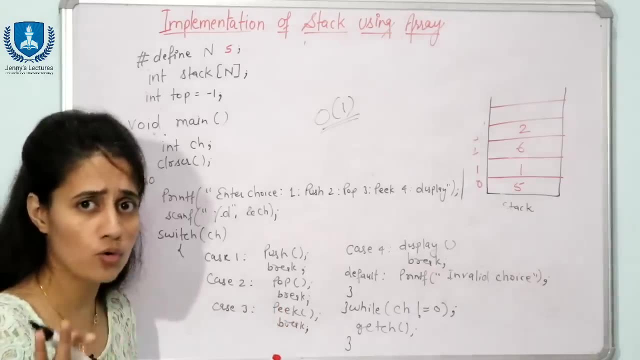 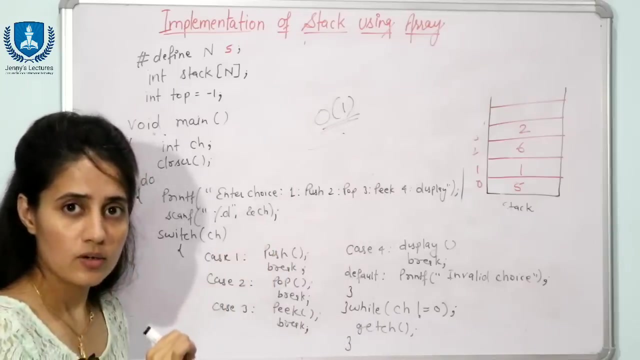 right, because, as you have seen, in all the push, pop and peak operations we haven't used any that for loop fine. so that is why the time complexity is order of one- fine, maybe for searching or for displaying the content it is order of n- fine, but for these operations 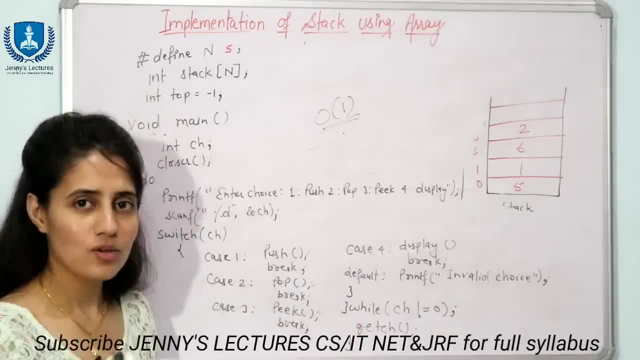 it is order of one one only, fine, so now i will see you in the next video. till then, bye, bye, take care. 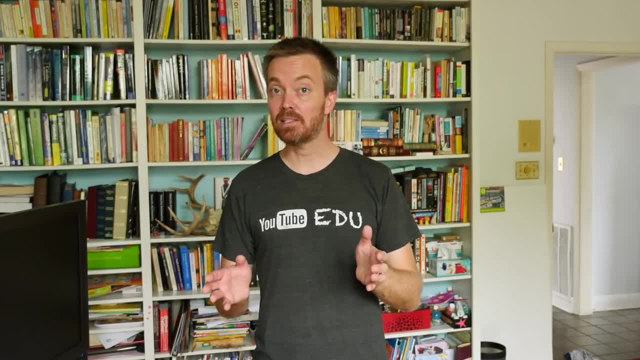 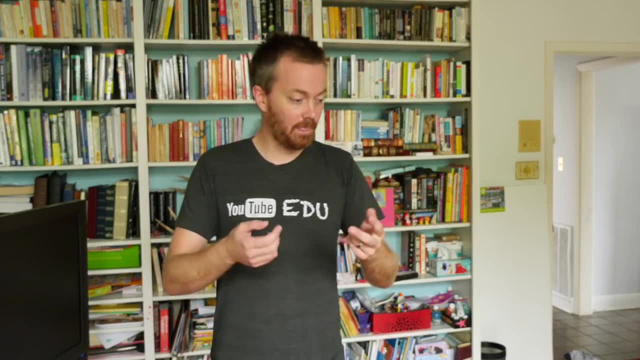 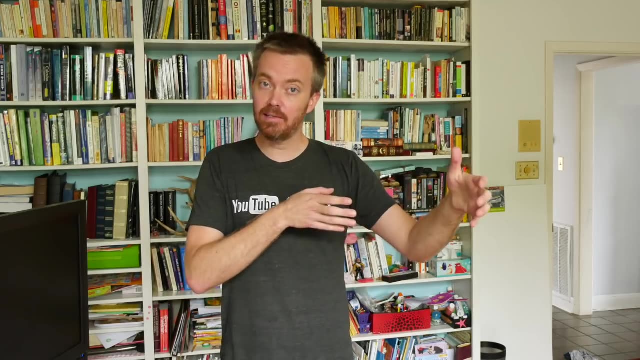 So in this video I want to talk a little bit about the mathematics involved in our current form of encryption. So the basic idea is you publish two numbers and these are what are known as your public key, and it's akin to what I discussed in the first video. So in the first video I said: you know you can go.